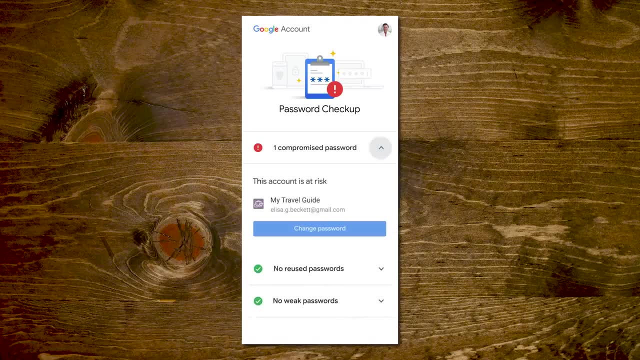 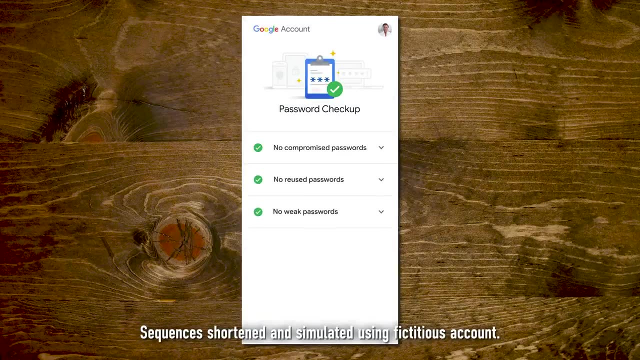 all within the security of my Google account. I even like to take it a step further with Google's password checkup, which strengthens saved password security and lets me know if any of my saved passwords have been compromised and need updating. It's also free. 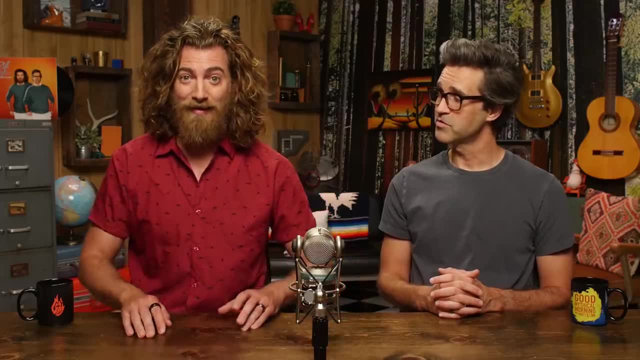 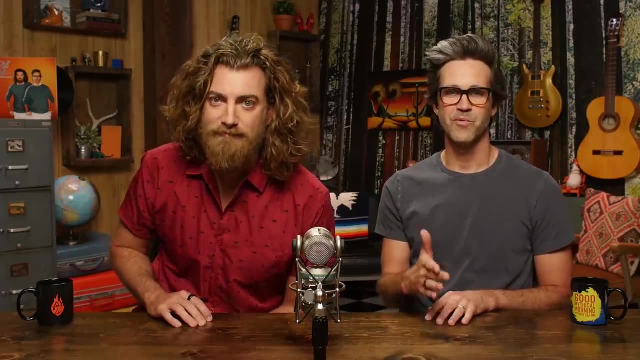 And you know free, that's my favorite four letter word. Well, I thought that was beans. Nope, bean is my third favorite, right behind free and wood. Okay, Your private information is valuable and weak. duplicate passwords are easy to hack. 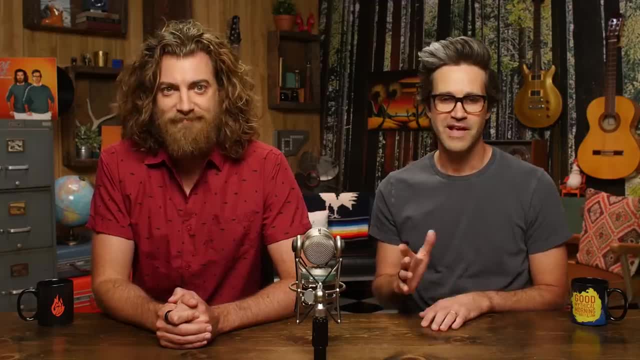 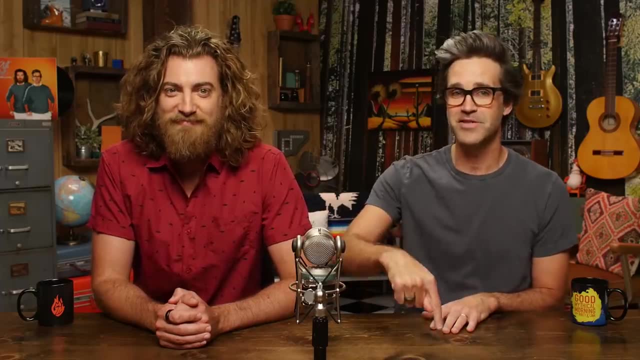 I tell my family this all the time: Yes, mm-hmm. For example, what I love for all of my online passwords would just be the sound that Chase makes when he tears an apple in half, plus the year that I tried my first peanut butter cup. 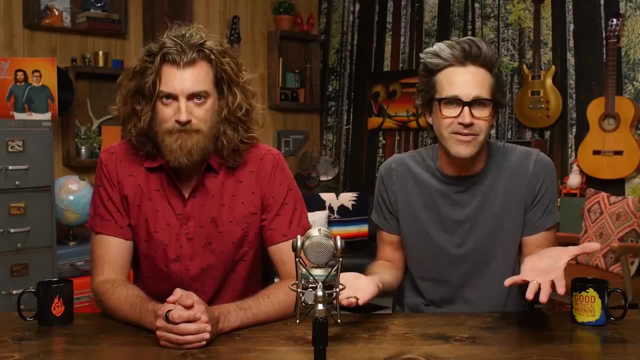 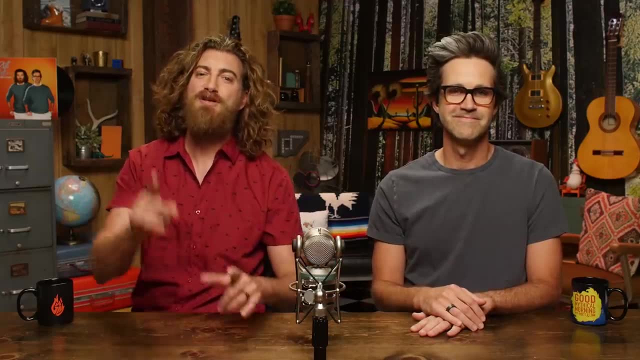 Of course I would, but that would be too easy for anyone to figure out, Right, because it would be: ah, 1983. See, Yeah, Google securely stores your passwords, so they remain private to you And you can use a password checkup. 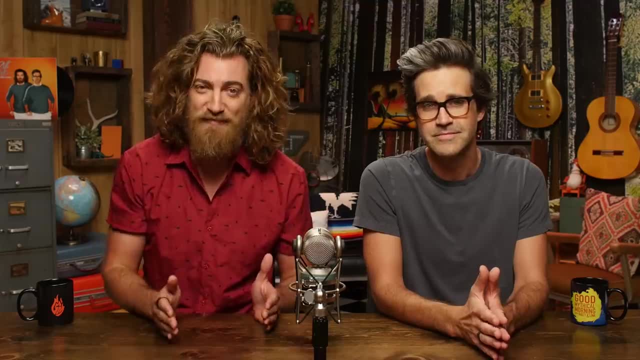 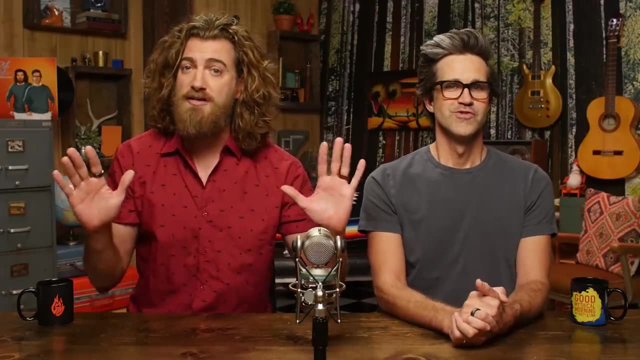 to strengthen the security of your saved passwords, to keep your personal information safe. Thanks to Google for sponsoring that part of today's episode. Now we're gonna conduct some science experiments without instructions or adult supervision. It's time, for The Idea of Direction Simply Disgusts Us. 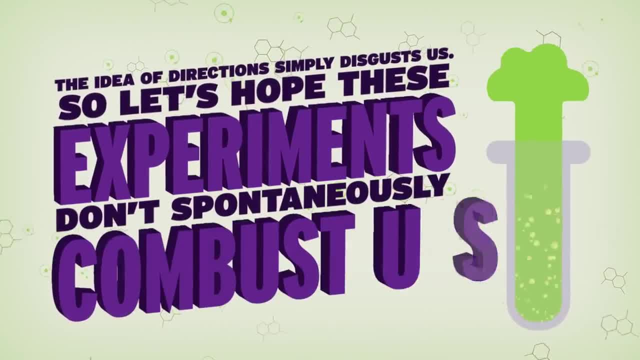 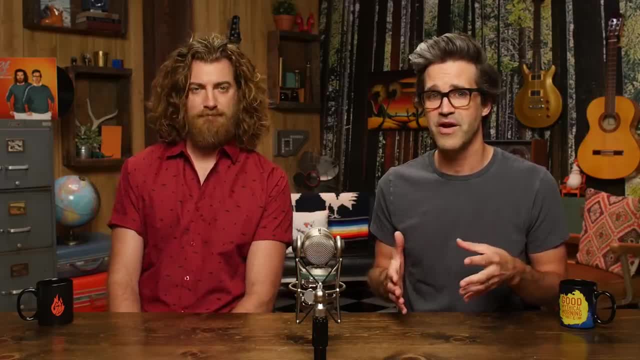 So let's hope these experiments don't spontaneously combust us. We're gonna be given some items to conduct a certain scientific experiment and we have to try our best to figure out which of those items we need and how we need to put them together. 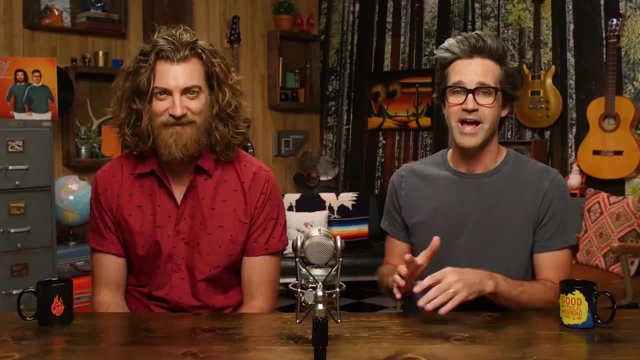 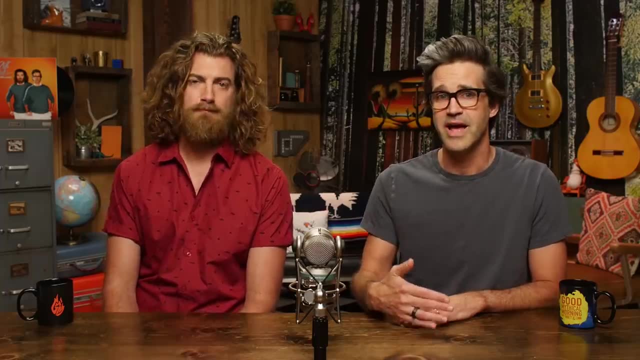 in order to get a specific crazy scientific result, And there's gonna be some fake-out items thrown in the mix to try to throw us off of our game. Now we're gonna start with 50 points and if we can't put the right pieces together, 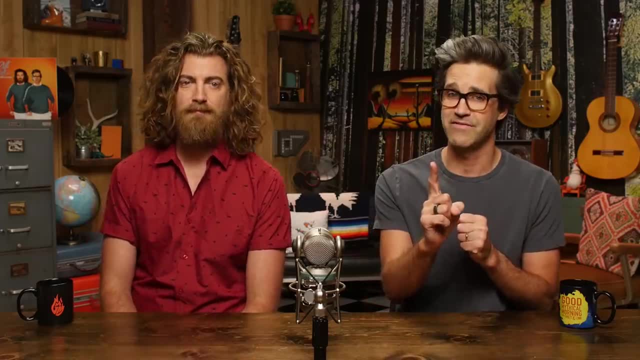 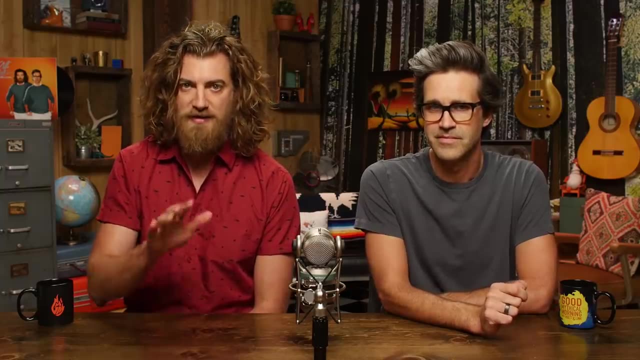 in order to make this science happen, we can't ask for lifelines, But all these lifelines cost points, and the more helpful a lifeline is, the more points that it costs. We got 10 minutes to figure out each experiment. 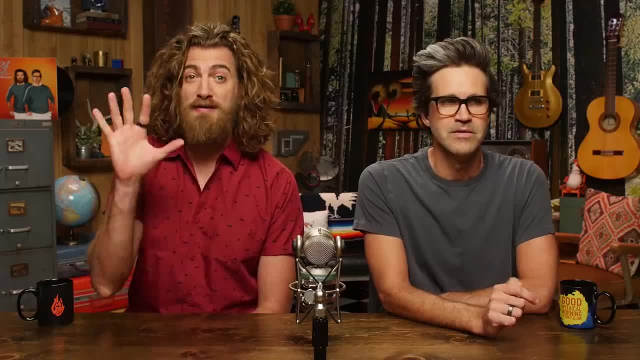 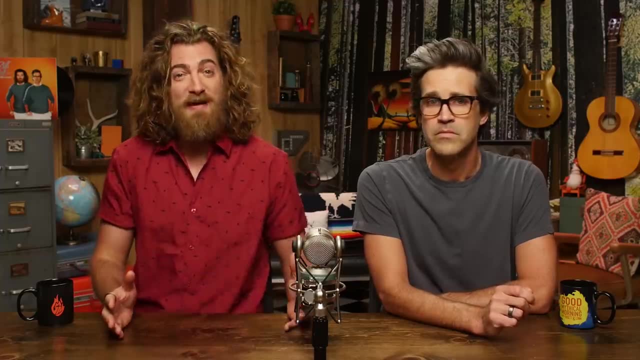 and if we still haven't cracked it when the time is up. that's a five-point deduction. What we're trying to do is, at the end, still have 25 points or more, because that means that we will win participation ribbons. 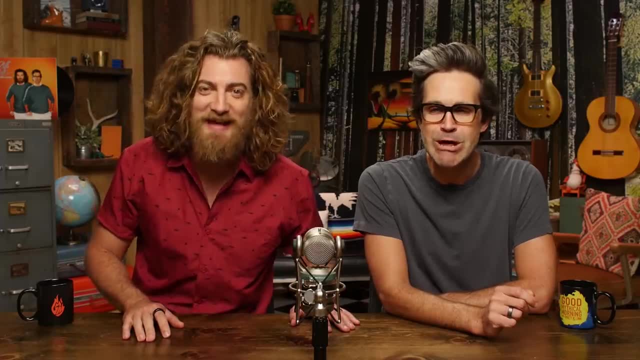 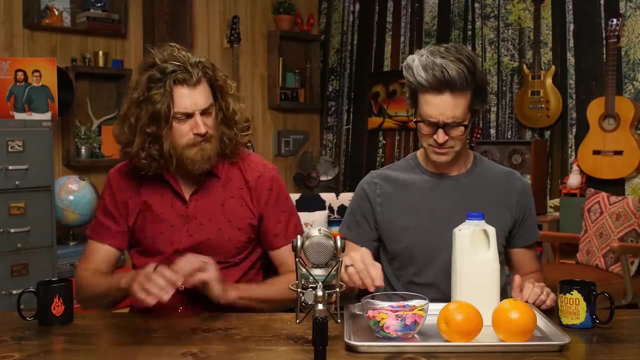 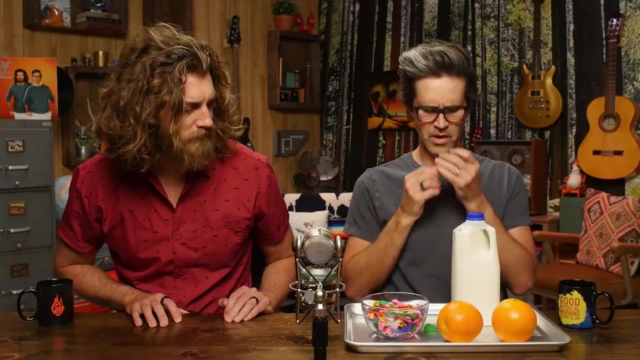 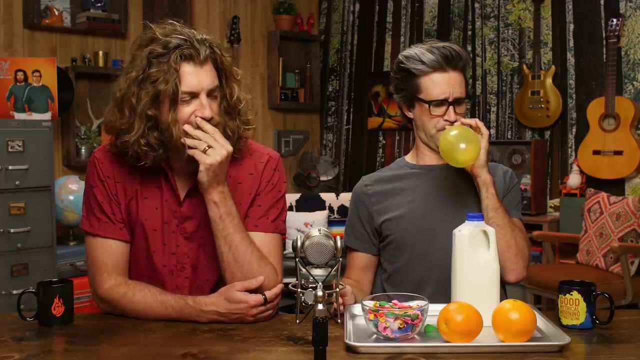 and a special message from Senior Scientist Chase. It's a special message. In this first round, you will use some combination of latex, rubber balloons, a carton of milk and oranges to achieve an unexpected result. As a reminder, one of these items is a decoy item. 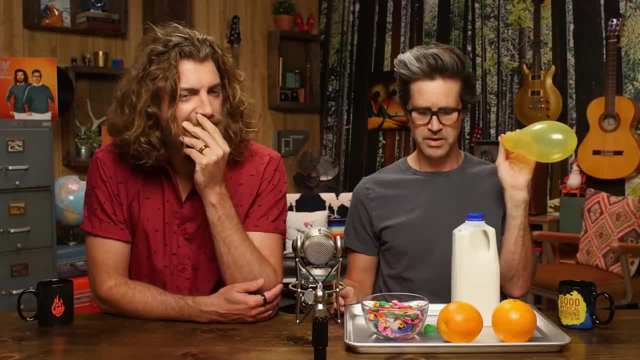 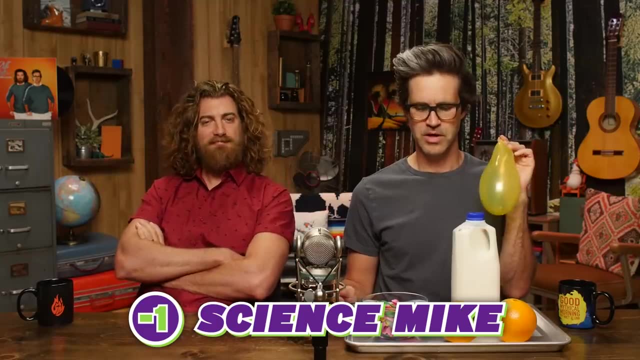 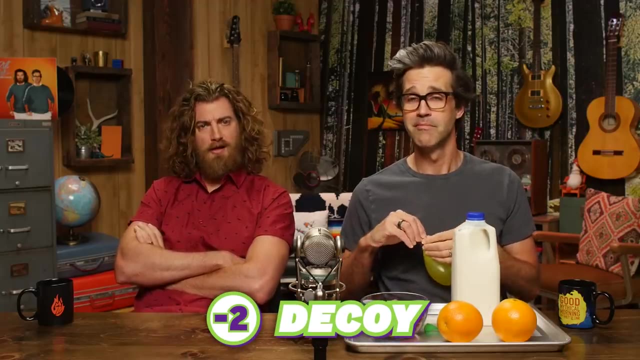 that you do not need, And your lifelines are as follows: A message from Science, Mike, about the scientific principle at play, which will cost you one point- Oh, that's not a lot. I tell you which item is the decoy. 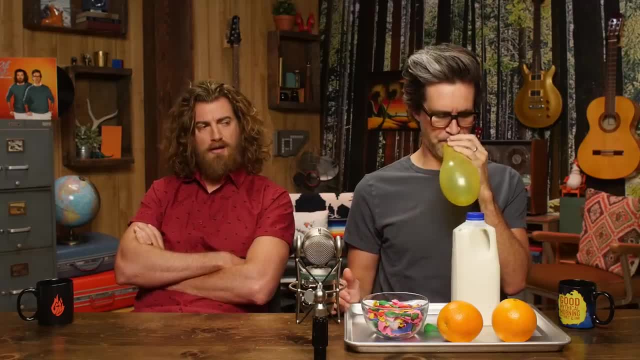 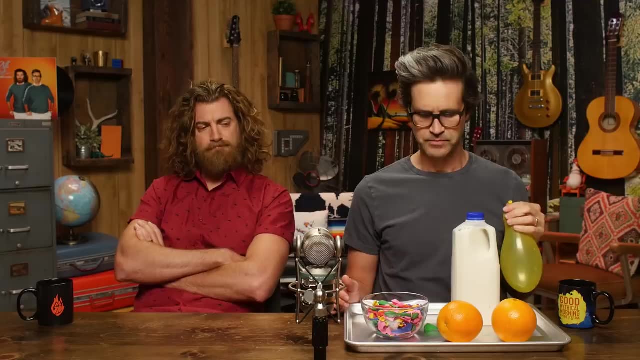 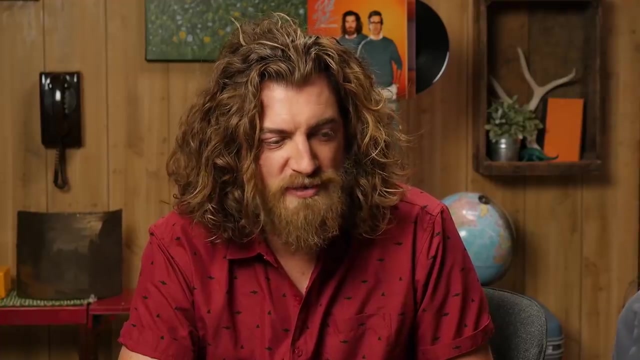 This would cost you two points. And I tell you what result you're trying to achieve and that would cost you three points. So with that, good luck. So if we remove the oranges, it's both oranges, obviously. Well, as a man whose thing is pouring milk, 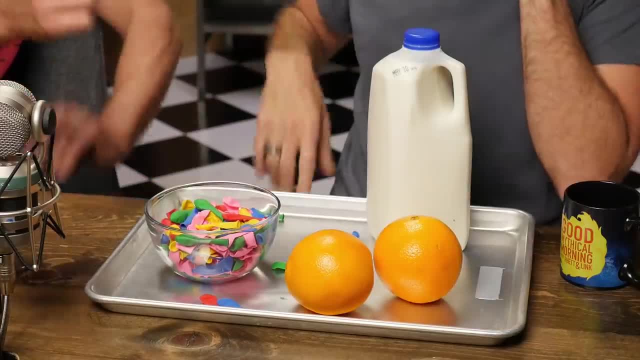 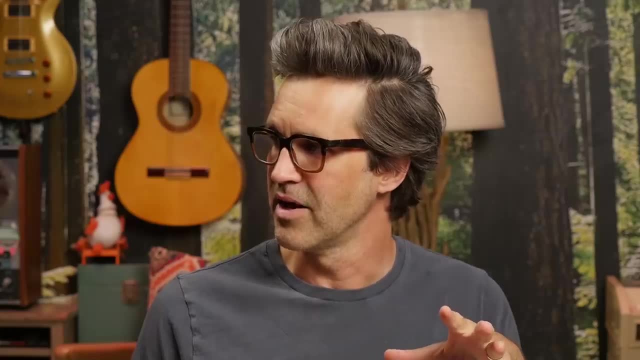 I really want to keep the milk so I can do my thing. You want to treat this like a bowl of cereal, don't you? This is gonna get blown up somehow. This is gonna get blown up. What else could happen? Let's get Science Mike in on this. 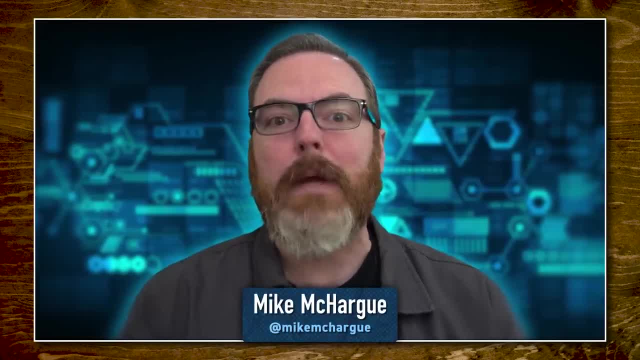 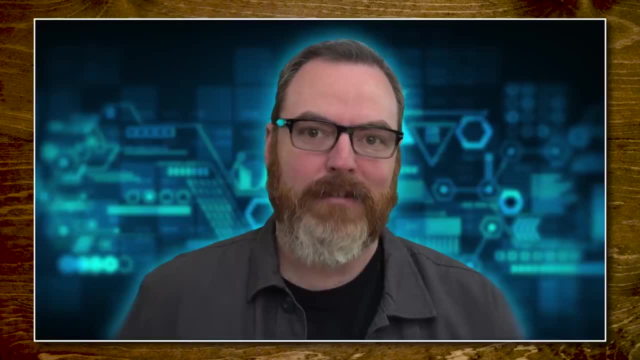 Yeah, just one point. All you need to do is find the right pairing of hydrocarbons. They're very alike, so you'd think they'd be great friends, but they can really wear each other out. I think we need to mix these two and see what happens. 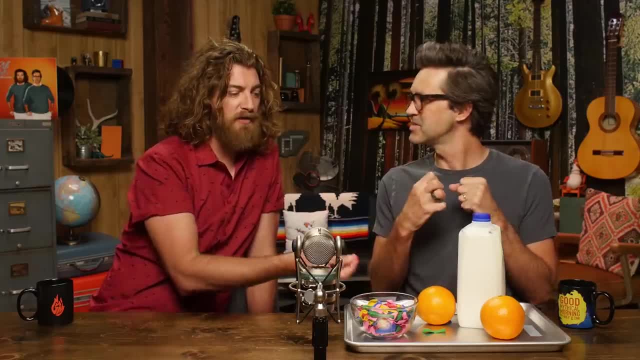 You think the balloons are going out, Based on what Mike said? yeah, because it was like two things that seemed similar And we're gonna be left with just milk and oranges. Well, I'm gonna put the orange juice in the milk. 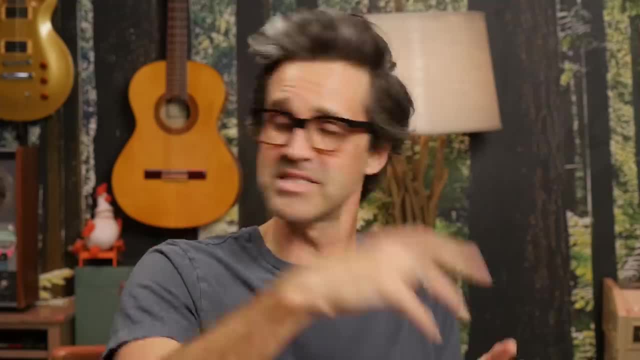 and I think that it's gonna curdle. I'm gonna put the lid on and it's gonna bust the lid off. Squeeze it in there. See this amazing reaction. that's gonna happen. There's no way that milk is going to explode. 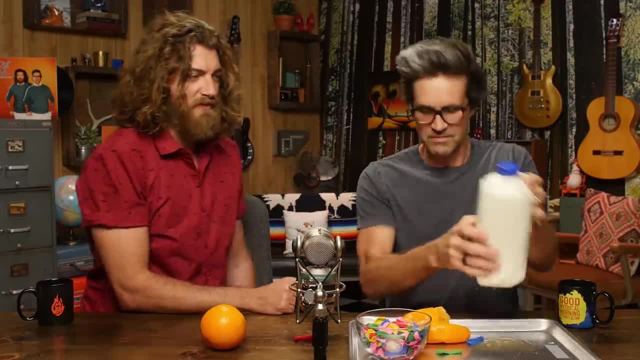 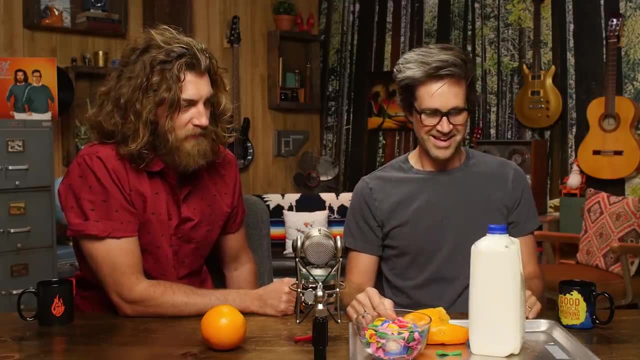 right here in front of us. They wouldn't do that, But I'm willing to go down this ride. Okay, Boom, It's not gonna bust out. Oh God, you just got orange juice in my eye. I think we gotta remove an item. 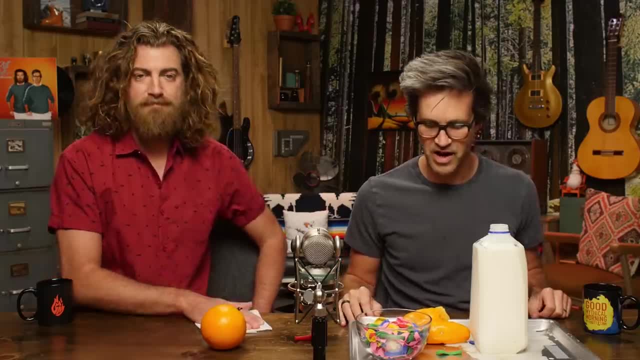 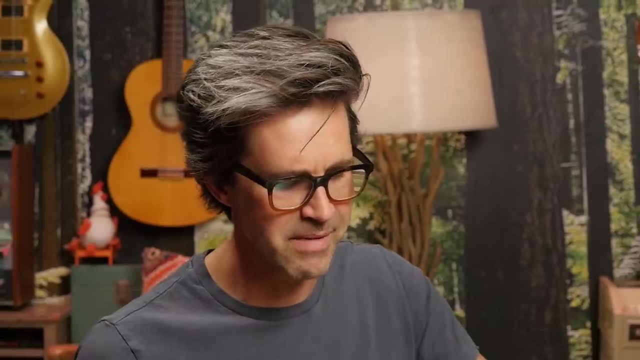 because there's only so many ways that these things can interact. Okay, Stevie, we wanna remove an item. You do not need the milk. Yeah, I'm not surprised. Well, what Mike said didn't make any sense. He said it would wear it out. 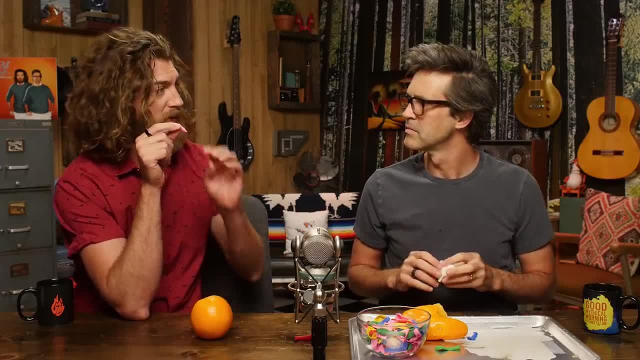 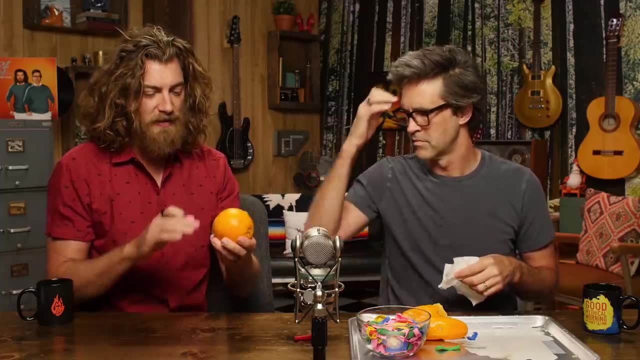 I think we have to blow up this balloon separately, and then I think we have to do something with the orange that's gonna make the balloon pop, because the acid from the orange is going to pop the balloon. Okay, let's blow up some balloons. 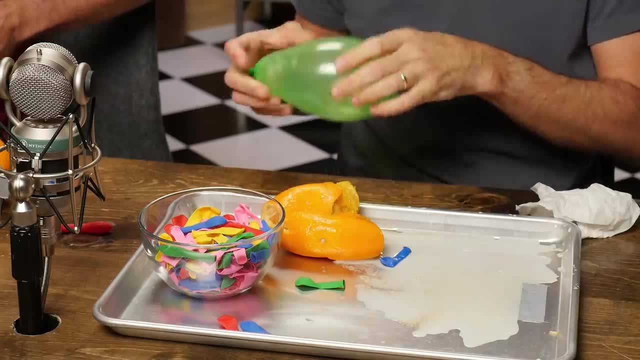 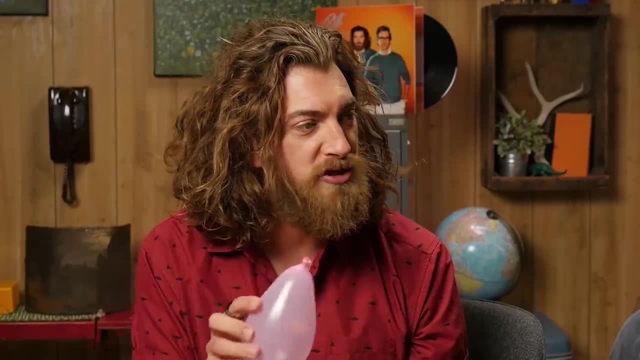 Pretty good, Good at that. Do you think that? then, rubbing an orange on a? You do it, man, because you're gonna look stupid. Oh, the juice should be inside of the balloon. You blow the balloon up, you get orange juice inside the balloon. 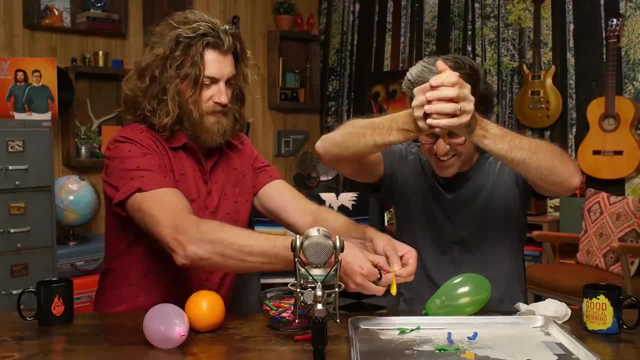 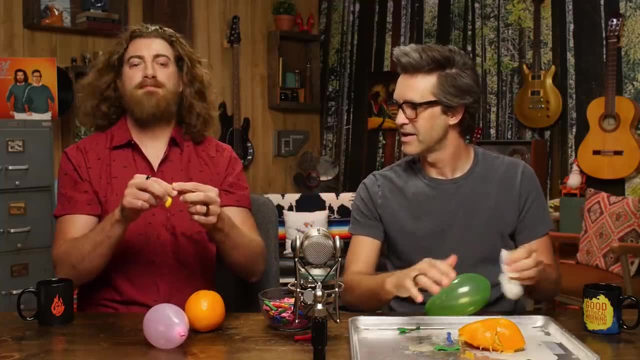 you shake it, you set it down and it will pop the balloon. You can get some juice in there. I don't think it takes much. Okay, Just a little bit Now. It goes a long way. Now see if you can blow that up. 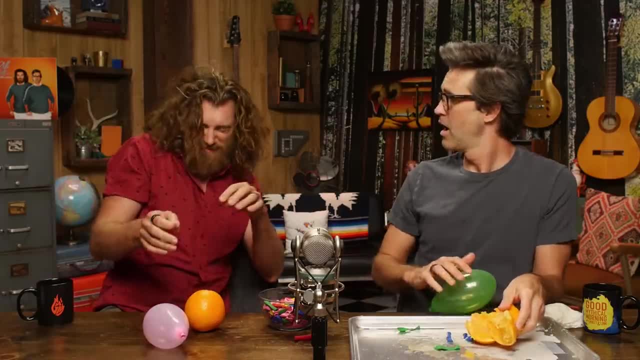 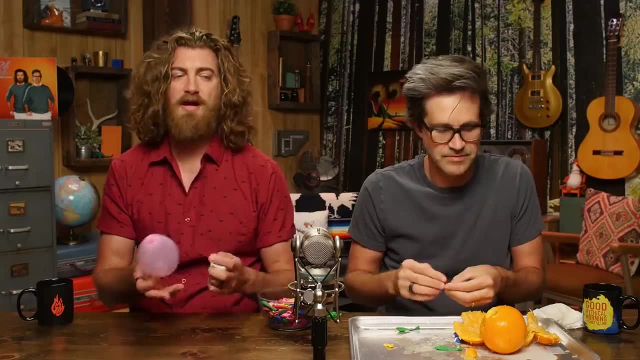 because what I think it is, I think it. Oh yeah, that was it. I'm starting to hate science, Stevie, Do we need to? We need to get. We're gonna have to go with her third thing. Okay, you gotta tell us what we're trying to do. 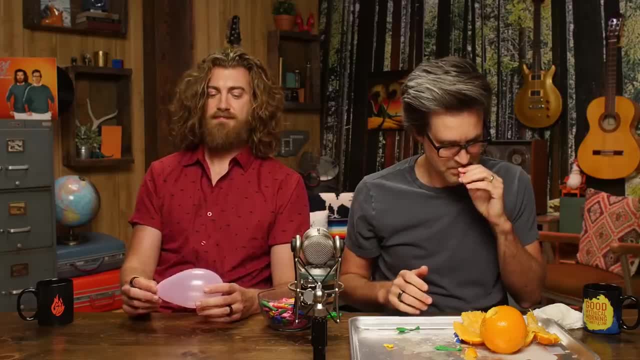 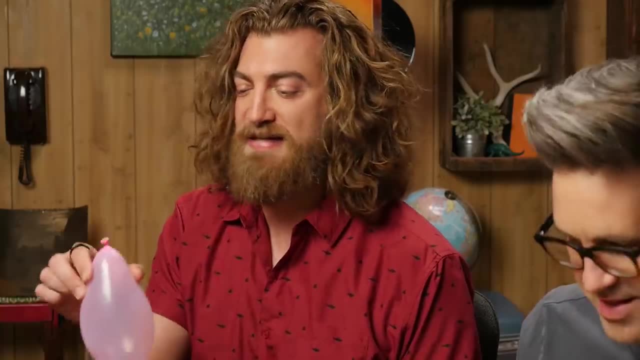 I will say this: You have already said what you're supposed to do, but you have not Done. There's orange juice that needs to be inside the balloon, and then you shake it. I think that's what it is, So let's do that again. 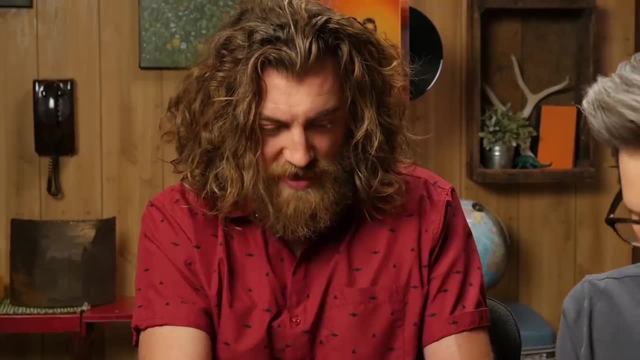 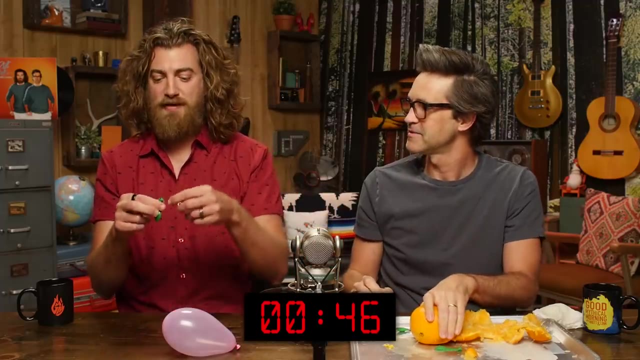 and I won't blow it up so big. And I've got a hole in this one now, Yeah, squeeze it right out of your hole, right into this. Okay, Juice is going in. Now what? Now I blow it, But I can't blow it too big. 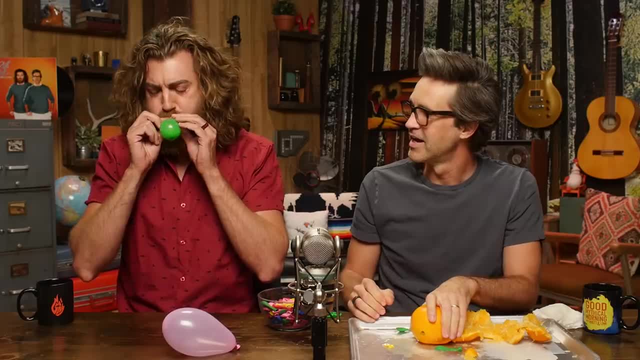 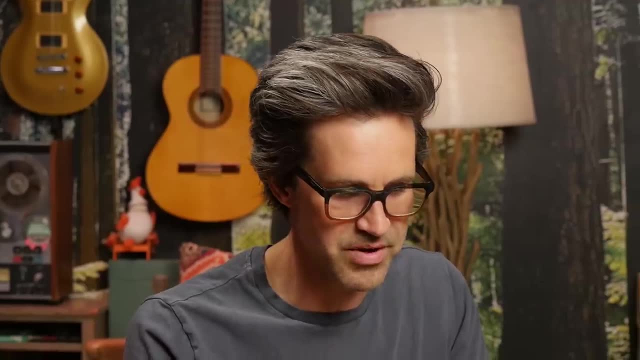 45 seconds. Come on. come on, Just a little bit. No, that's not big enough. A little bit more, a little bit more. No, last time it exploded really early in the process. Put it inside. You wanna put it in this hole. 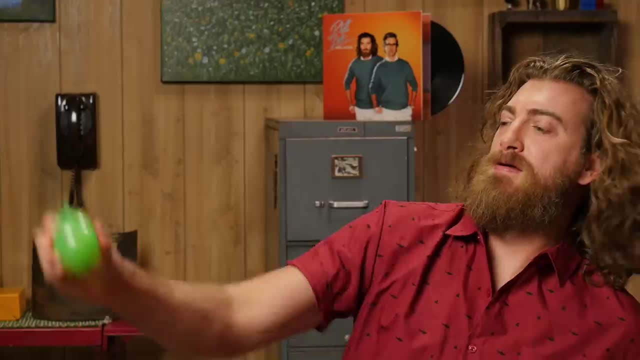 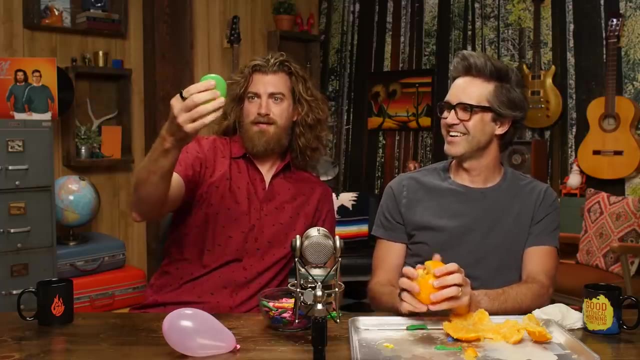 Maybe it goes in here. Okay, now I shake it 15 seconds. Ah, dang it. Come on, that ain't doing nothing Here. put it in here. Put it in here. Oh yeah, look at it, There you go. 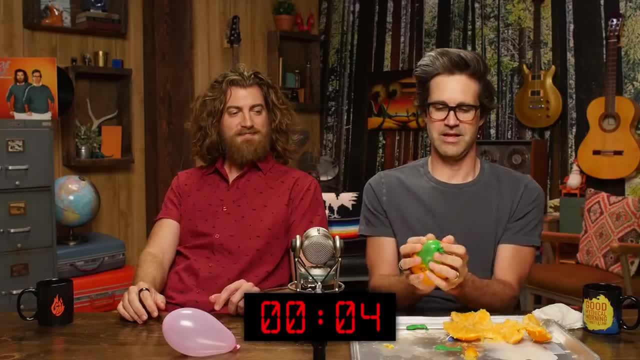 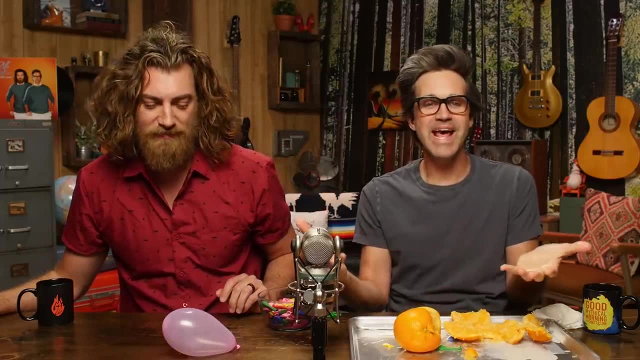 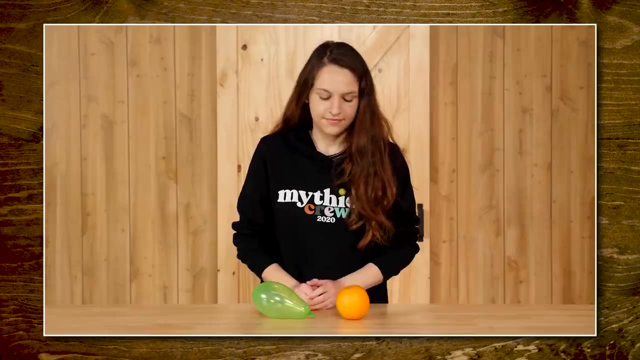 Now squeeze it hard: Five, four, three, two, one. We did it, Man, What is it? You guys were so close, but you didn't get it. Let's cut to a close. Here's a clip of Caitlin showing you how it's done. 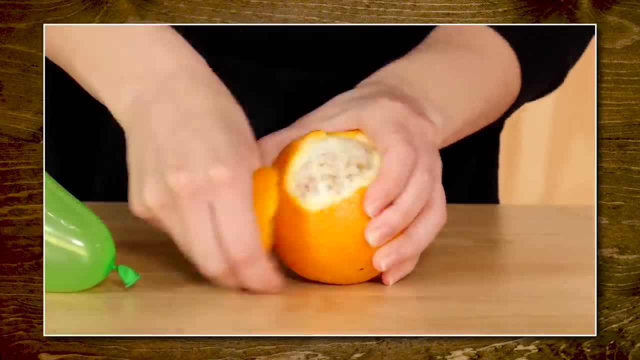 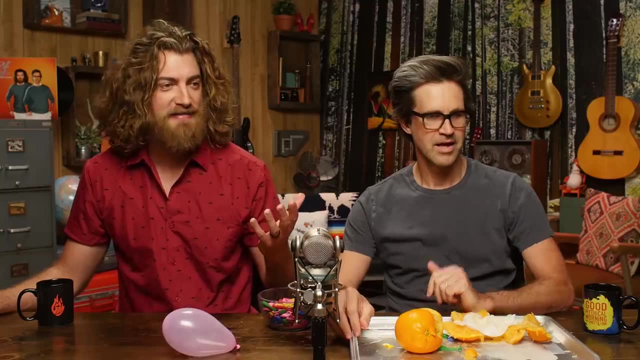 Oh, that music's horrible. Oh See, it wears the balloon out. It's the very first thing that I said, and then we never went back to it. What, Mrs Wizard over here? what did you do? Yeah, so it turns out. 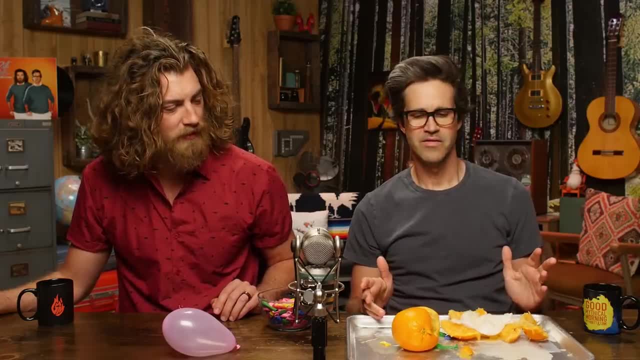 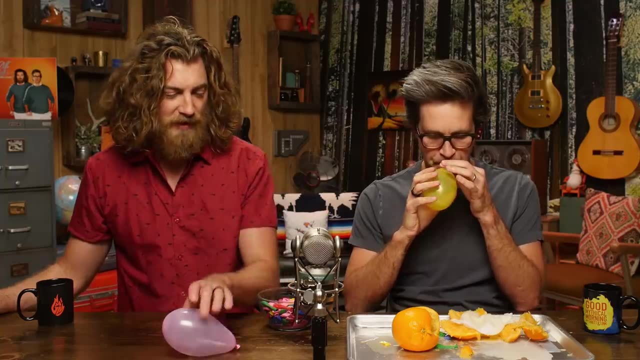 You just put a little juice on a balloon, Not the juice. Orange peels contain a hydrocarbon compound called limonene- Here I've got one already- And when limonene oil comes in contact with another hydrocarbon like rubber, 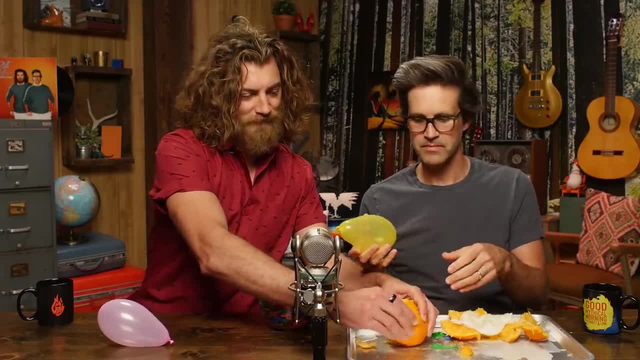 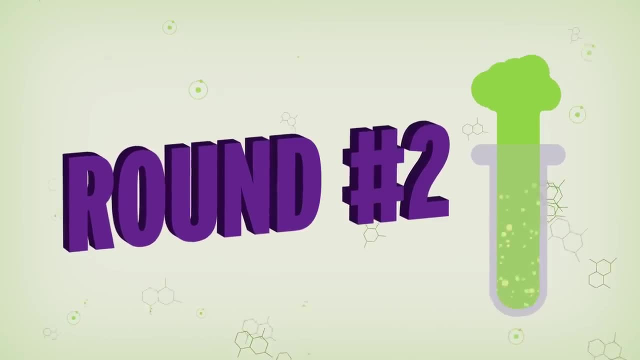 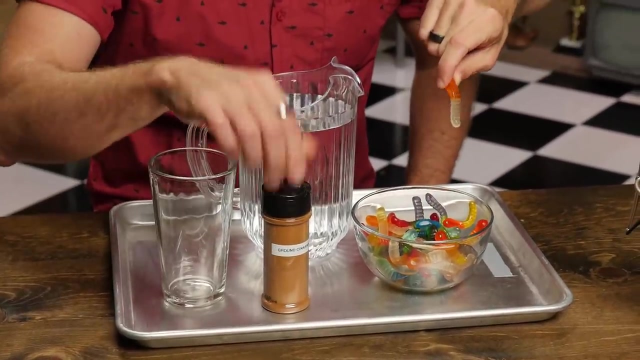 the rubber dissolves, which weakens the balloon and causes it to pop Hydrocarbons. see, So you said it, You just didn't ever really do it. This round, you'll use some of the following items: A glass gummy, worms, water and ground cinnamon. 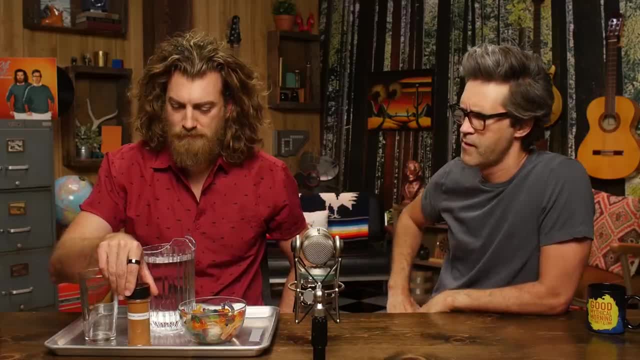 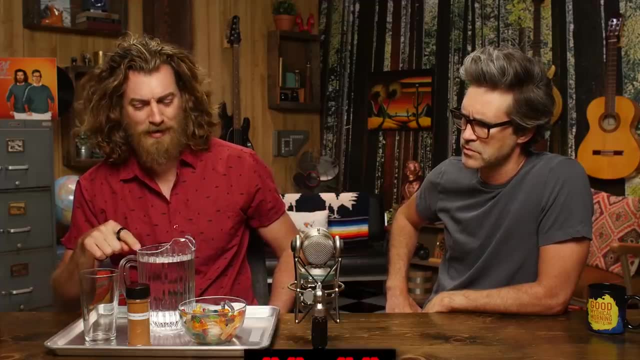 to reach your surprising discovery: Your lifeline's here. Your lifelines are the same as round one, so your 10 minutes starts now. A pitcher and a cup are the same thing. Yeah, I'm gonna say let's not use the cup. 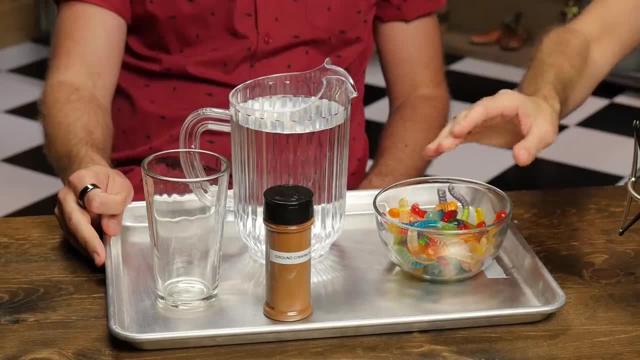 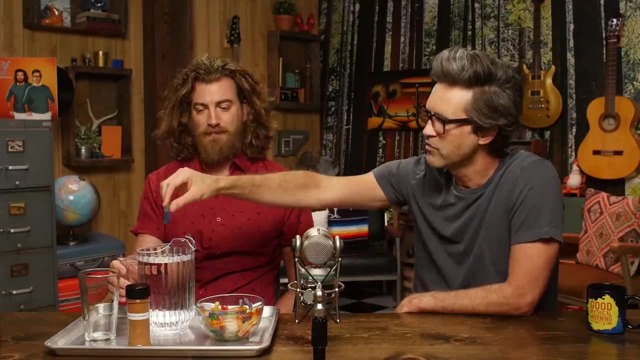 but if you mix, if you create a paste with the cinnamon Of cinnamon water, Let's do that. You know what we don't need. We might not need the water Or what if we don't need the cinnamon and you just wanna make worms swim? 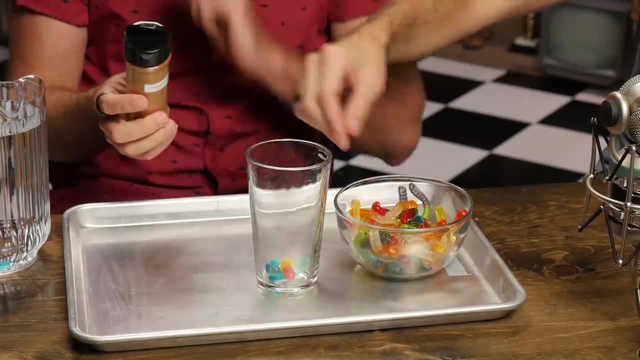 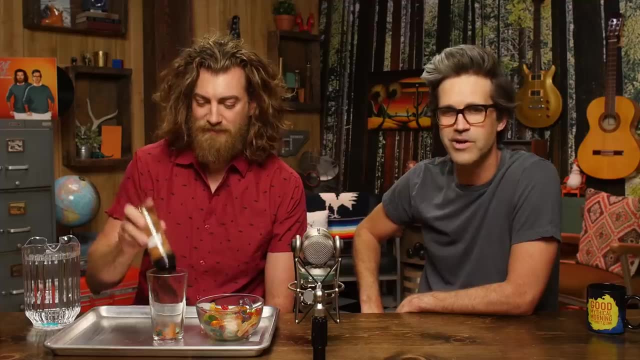 Put some worms in there. Okay, I'm gonna say some worms. if we're wrong, We're gonna load them up with cinnamon, Believe it or wrong. but Can we use our own spit? That would be an item. Okay, so you're putting cinnamon on gummy worms. 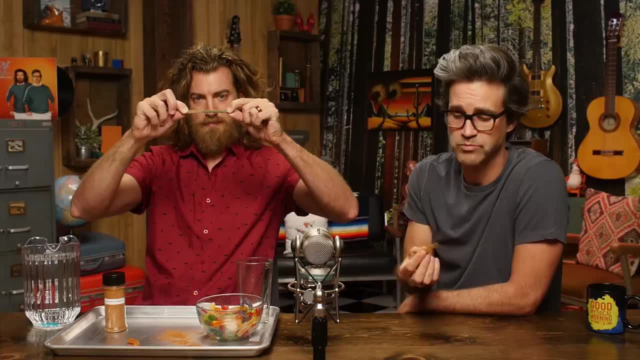 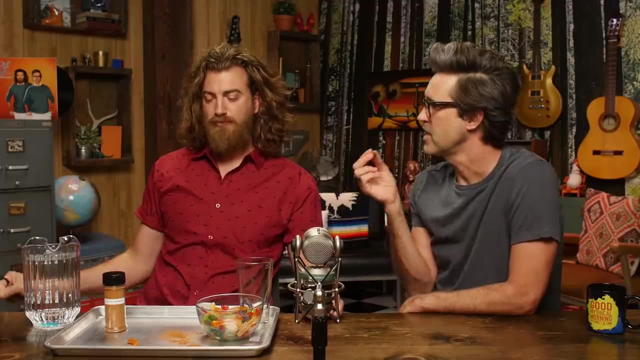 It can't be this simple. There's nothing, nothing gonna. Wow, they taste good Really. Yeah, taste one Christmas one. This is how you catch Santa Claus. You know what feels like the most distracting thing here For us just to eat these and not play the game. 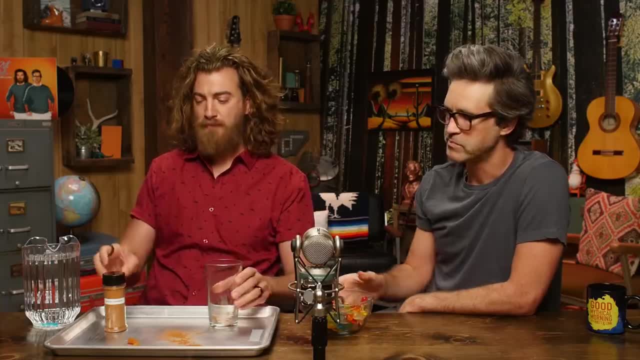 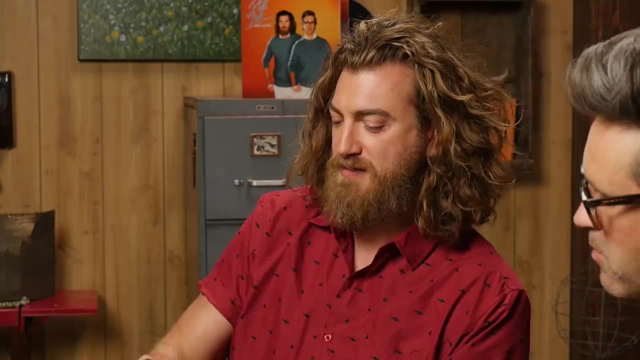 The worms. Let's forget about the worms for a second Mm, And let's make a cinnamon and water Paste, And then we're gonna rub it on ourselves and see what happens. You know what If you add water? That's enough. 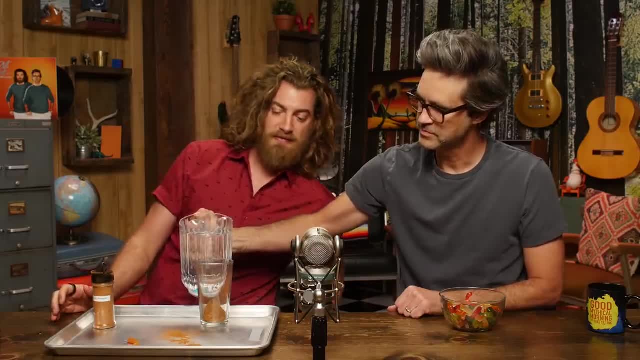 To cinnamon. you know what happens. Don't add much, Make a paste. Now what? Now put your hand over the top and shake it. Oh no, you do that. You're like a bartender man. We're gonna have to get Science Mike in on this. 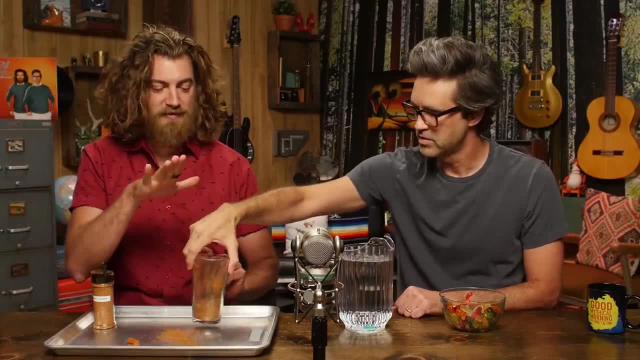 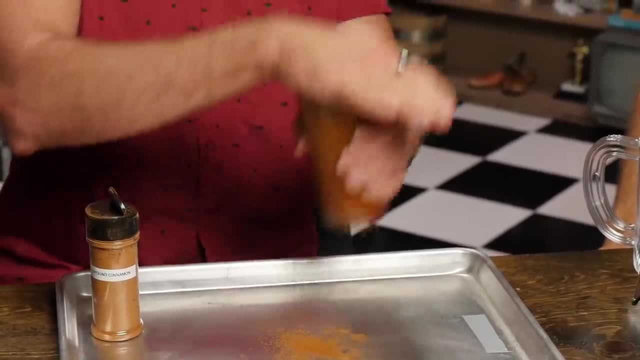 He's like he's trapped man. He's like he's trapped man. All right, let's see Science, Mike. The key scientific principle at play here is one that many may mistake as a fear. of water is one that many may mistake as a fear of water. 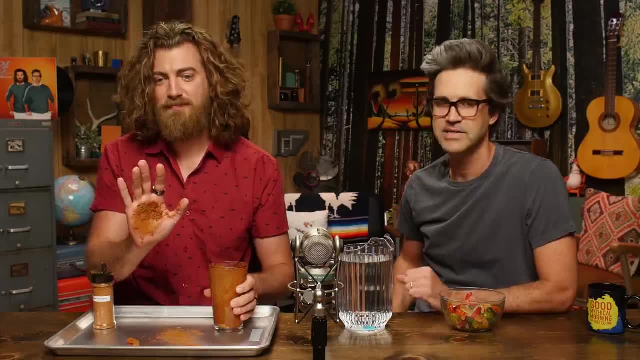 is one that many may mistake as a fear of water, but when you get down to the root of it, it's more of a pushing away of that ever so complex H2O, of that ever so complex H2O. Okay, The cinnamon and the water. 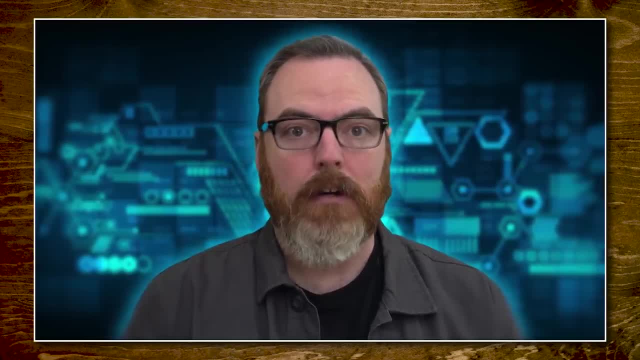 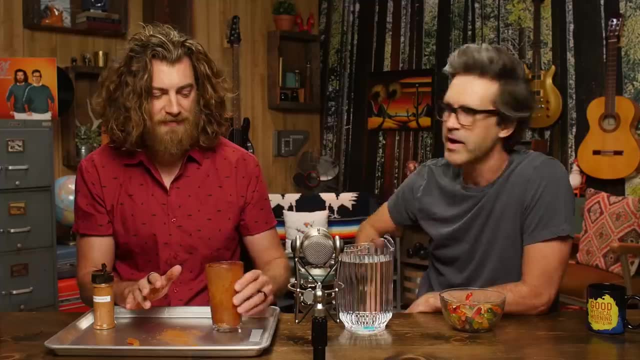 gotta do something crazy. All right here, all right Get. oh, we need a new glass, because this is a surface tension thing. because this is a surface tension thing, Okay, Okay, Okay, Okay, Okay, Okay, Okay. 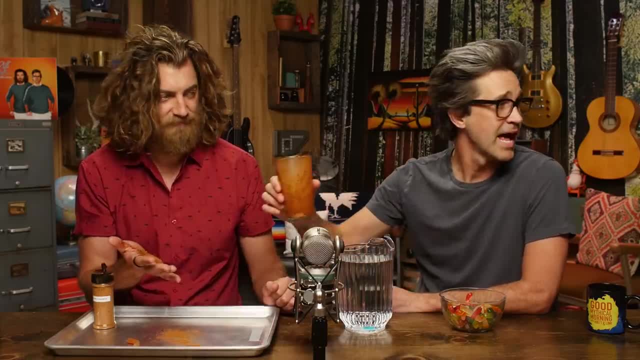 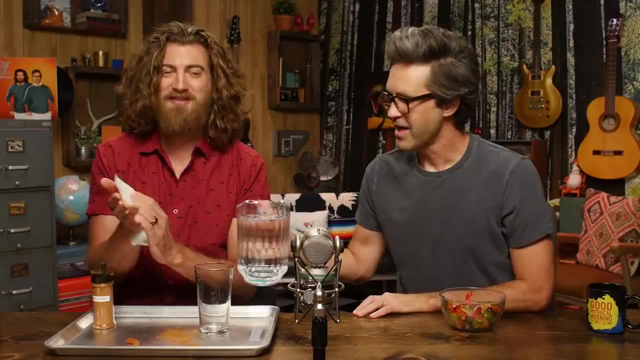 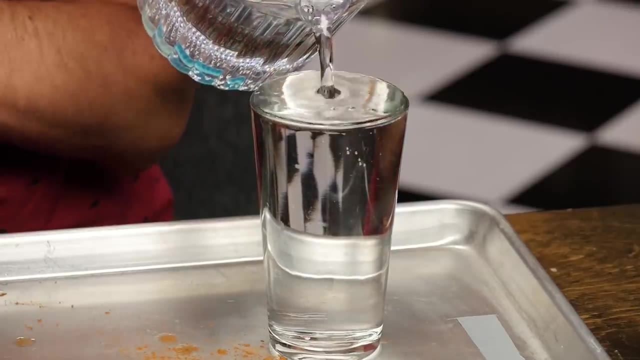 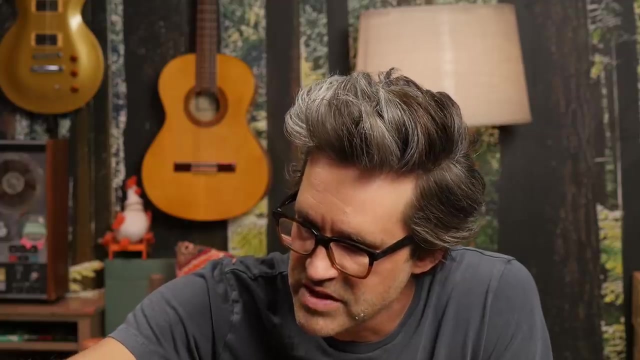 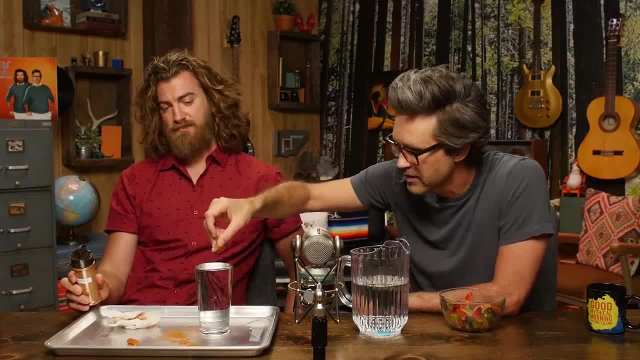 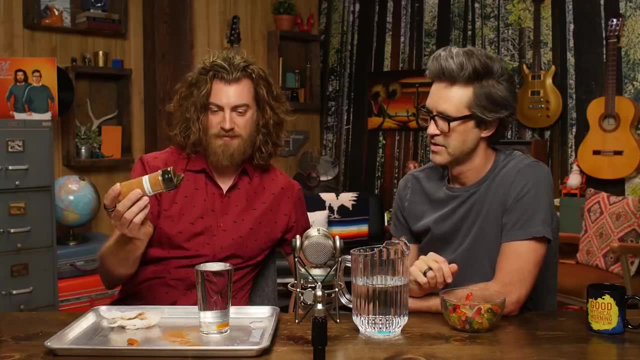 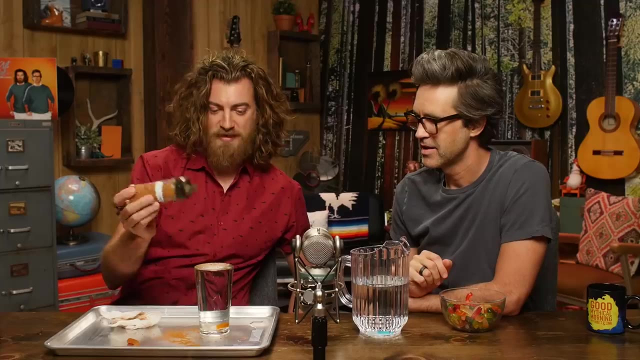 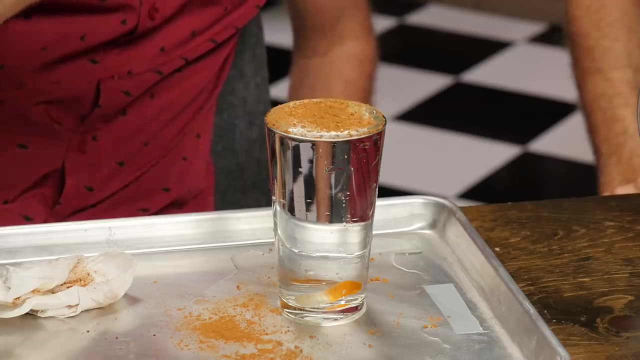 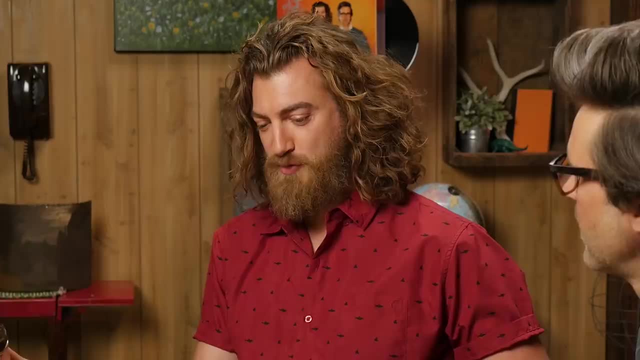 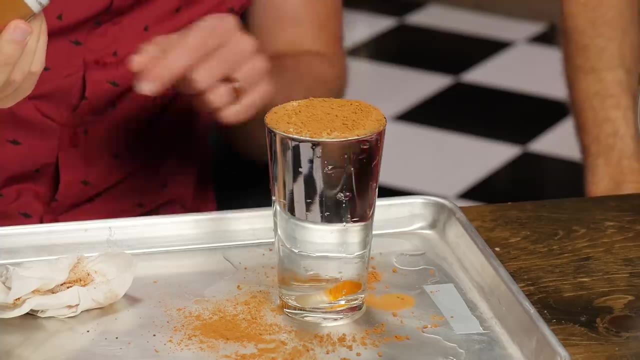 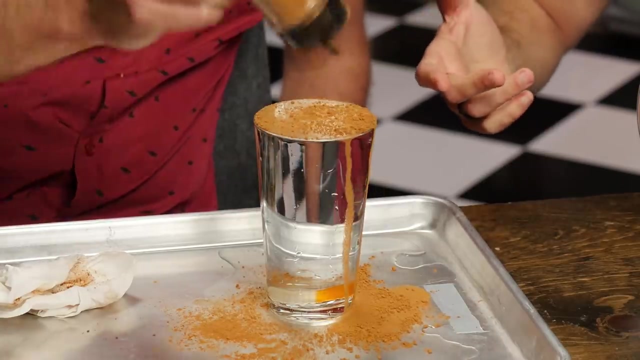 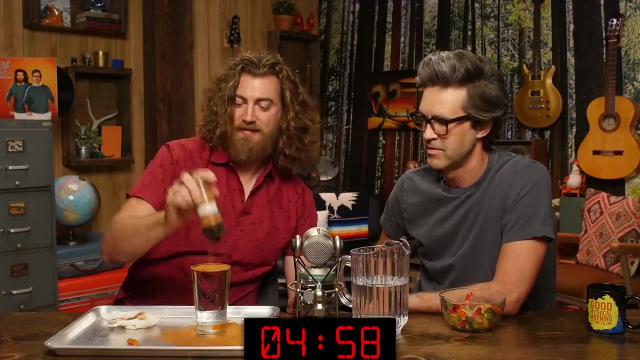 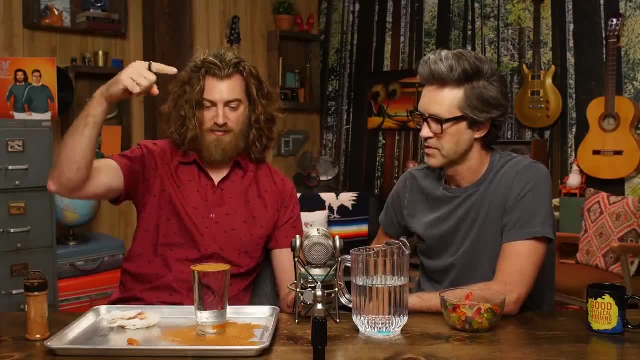 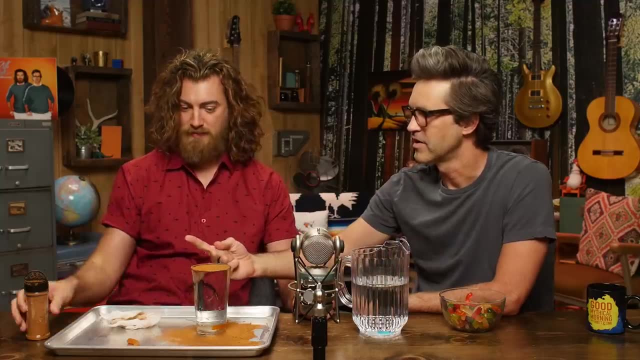 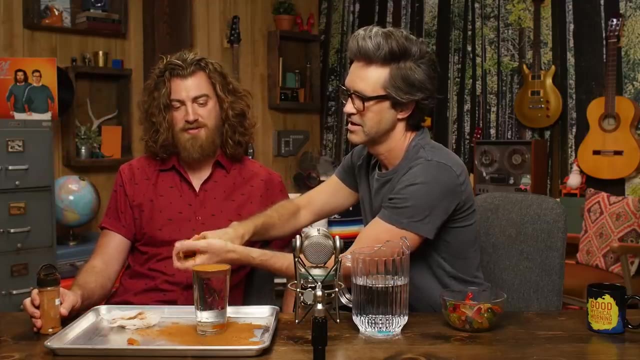 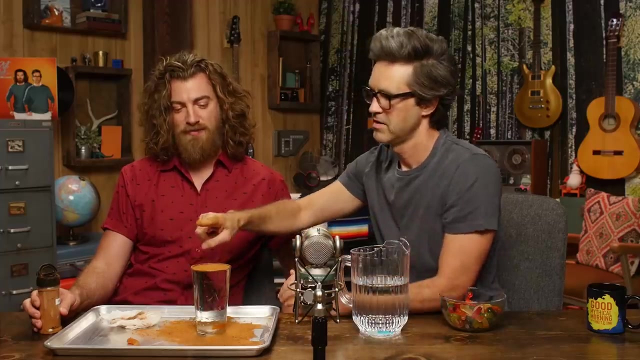 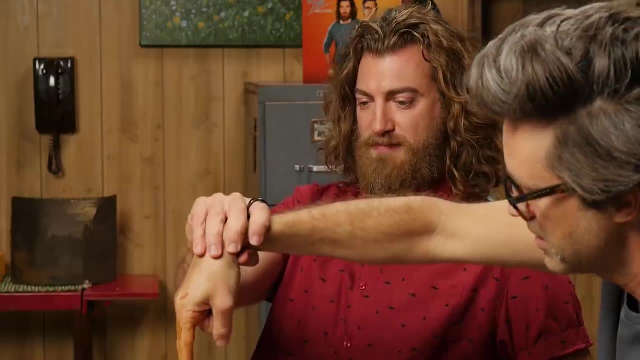 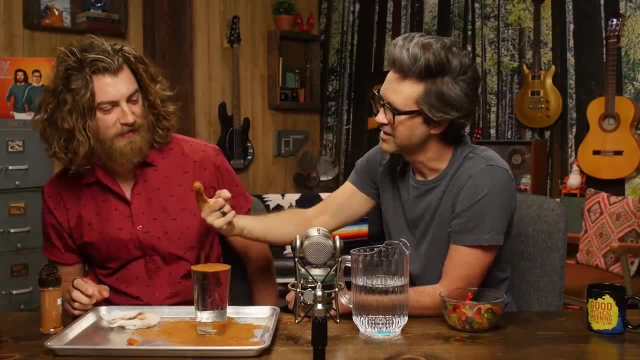 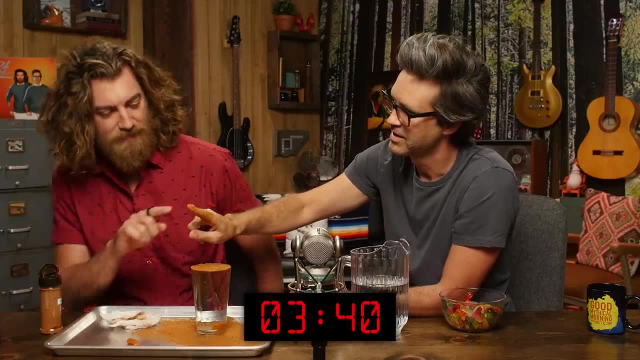 Holy mackerel, look what happened to your finger. Look at, it's kinda wet. That didn't work. It's not that wet, It's a little wet, though It's not that wet. Well, I'm gonna give it to you guys. 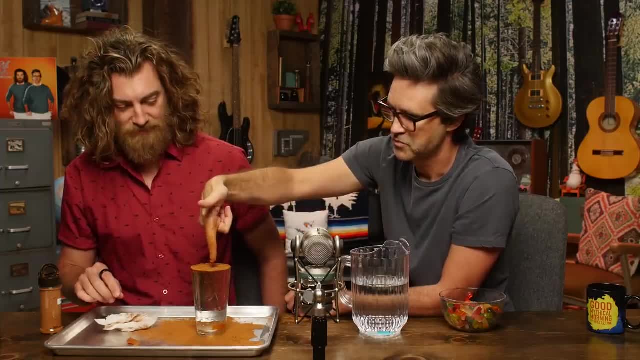 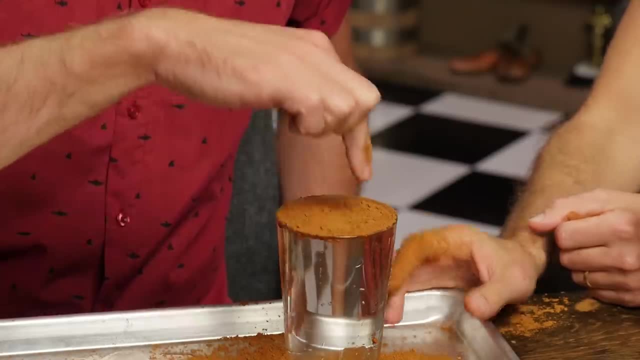 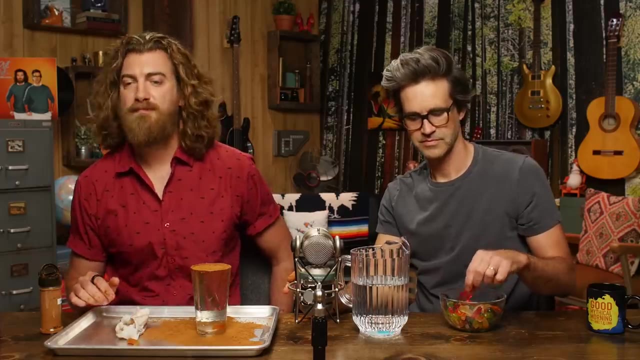 You went really deep, but, yes, you have everything in place that you need. So if you didn't go as deep, there you go. Yeah, so unlike happily hydrophilic substances like salt and sugar that easily dissolve in water, cinnamon powder is hydrophobic and does not dissolve. 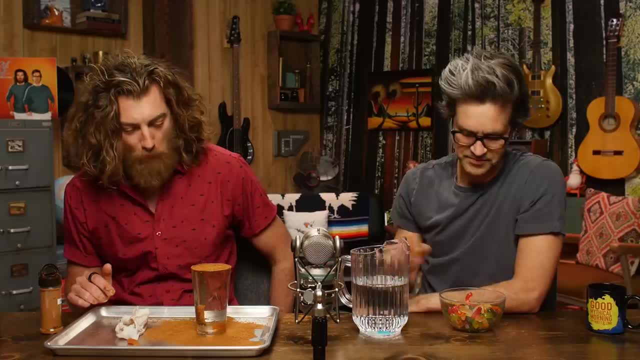 So when you stick your finger in, the cinnamon continues to stick to itself while still repelling the water, keeping it dry? Yeah, but have you had a gummy worm with cinnamon in it, Like Skid Night? Have you had a gummy worm with cinnamon on it? 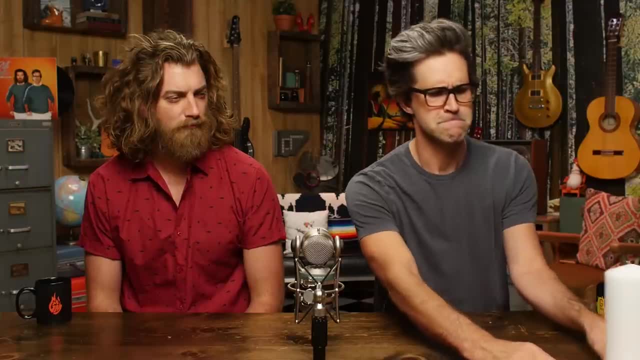 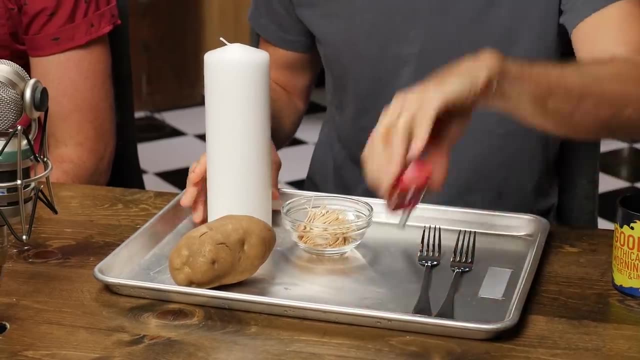 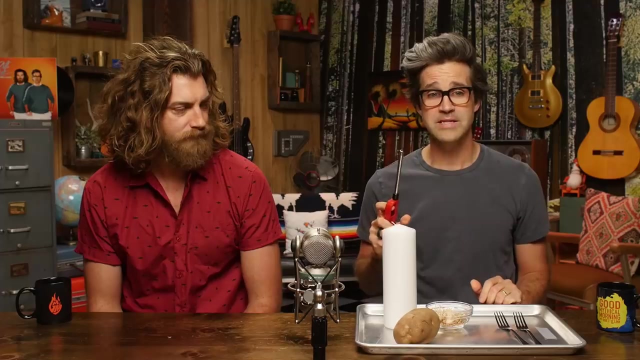 Because y'all should do that. All right, for this one. you will use a medley of forks, a lighter toothpicks, a potato and a candle to make some magic happen. Same lifelines again. Oh, not science this round. 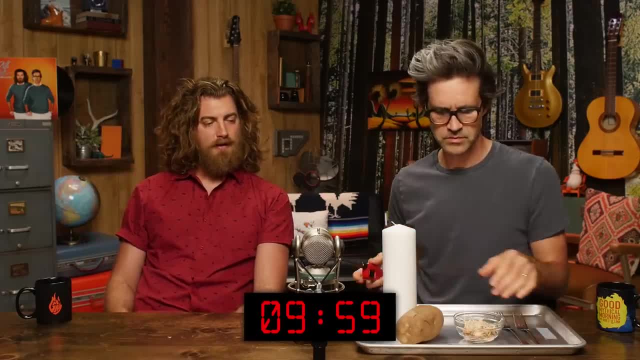 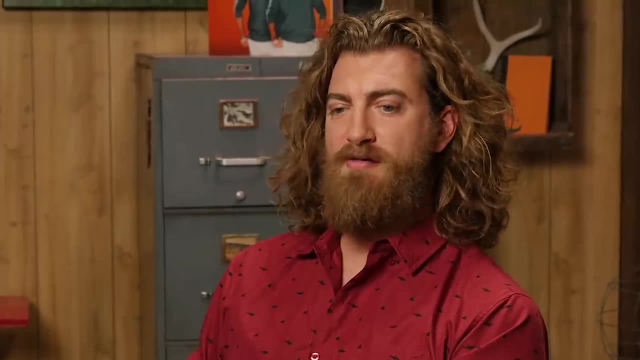 Pure magic, Pure magic, okay, And your 10 minutes start now. Obviously, something in the potato is flammable in some way that no one ever, no one ever imagined. I want to use fire, but I don't think we need the candle. 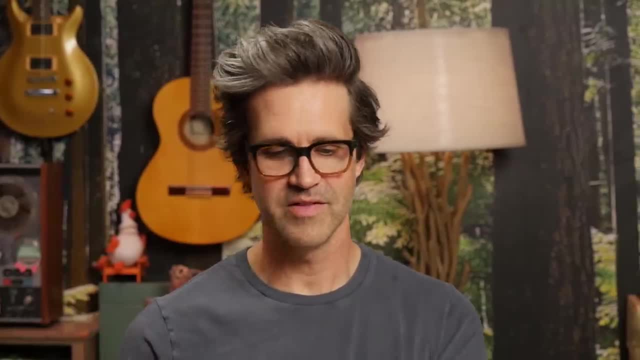 I feel like the candle is a distraction. That's what I was going to say. Right, because if you got rid of this, then what's the good of this? But what about-? But if you get rid of this, this is still really good. 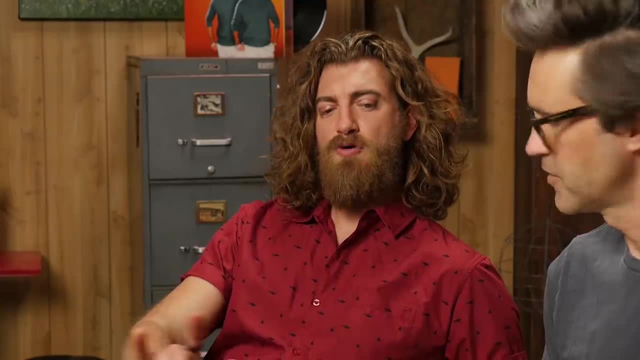 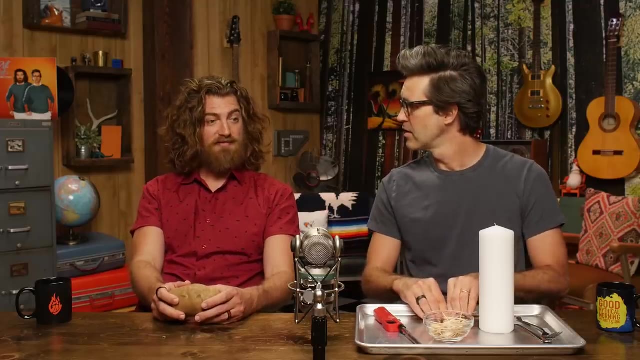 But do we need forks and things? Because everything a fork can do, a toothpick can do. You know what? Forget the potato. We can use our lifelines. by the way, Which one do you want to use? Well, I love seeing science, Mike. 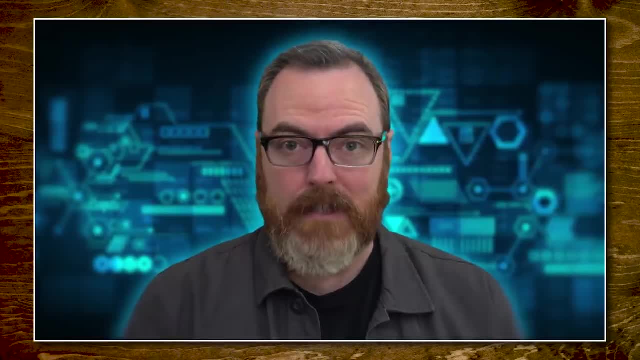 All right, let's see Mike again. The intersection of Newtonian physics and thermodynamics can create an almost magical series of things. The intersection of Newtonian physics and thermodynamics can create an almost magical series of things. The intersection of Newtonian physics and thermodynamics can create an almost magical series of things. 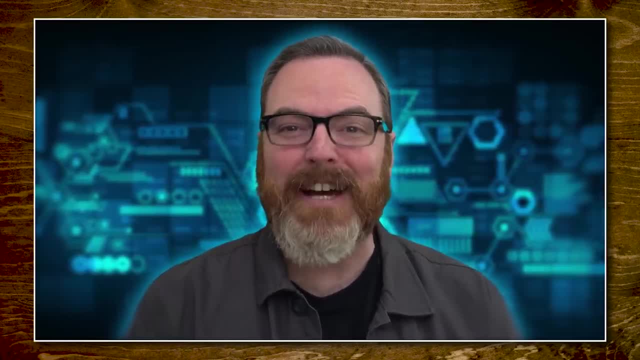 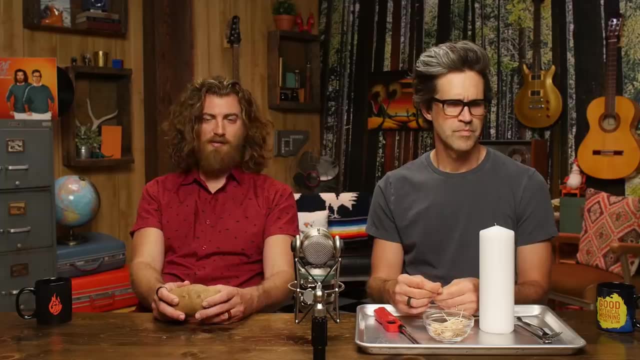 Even when you make it with your own hands and see it with your own eyes. it can be mesmerizing to see what the intricate balance of those two principles can do. Oh, come on, Mike. Who do you think we are Newtonian, and what? 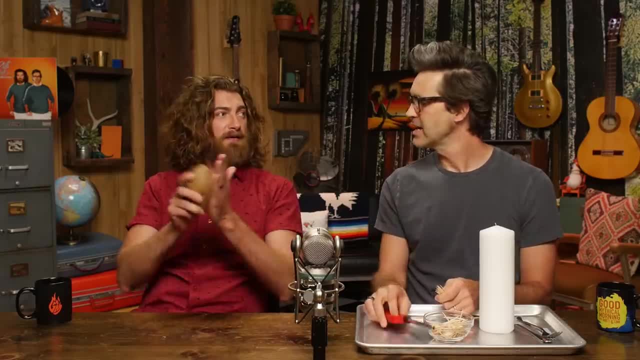 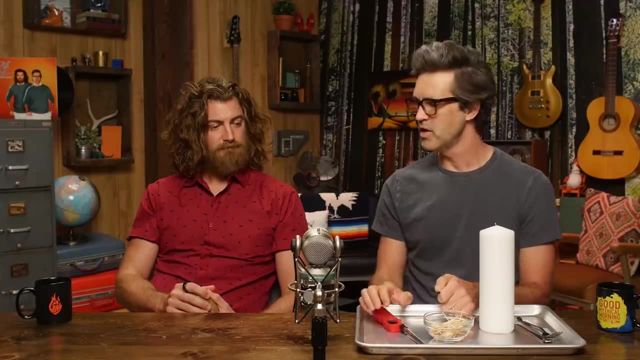 Thermodynamics, So physical things happening, Heat and like- Rubbing something to make something burn. I think- No, no, no, no, no, no. Rub the two toothpicks together. No, we have a lighter, But Newtonian is gravity, or like inertia. 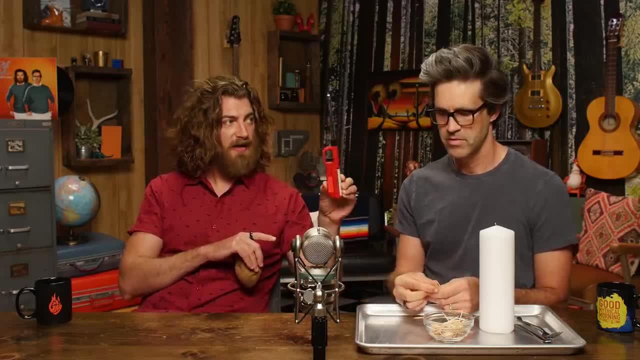 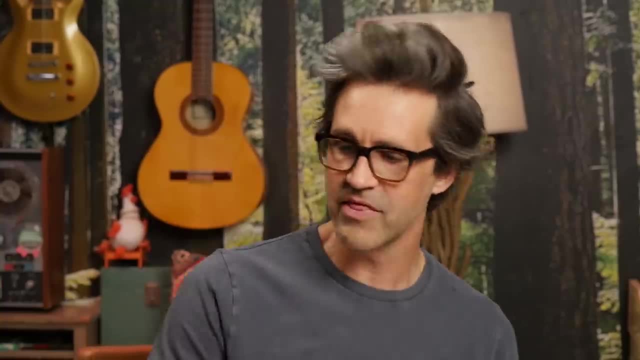 But Newtonian is gravity or like inertia. We don't need the lighter. The lighter's a distraction. The lighter is a cheat. We're going to make fire using just these things. We have to throw this really hard at the lighter. We just had to get 25 points. 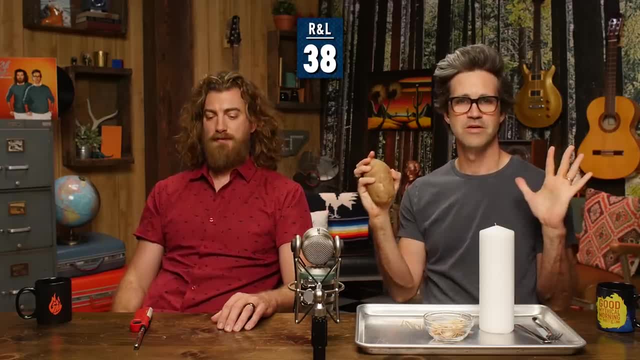 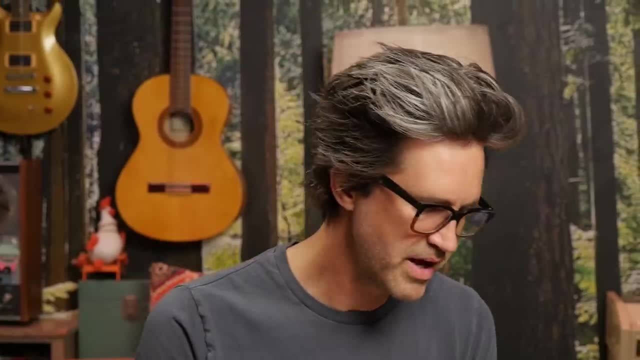 We should get rid of one of these items. All right, remove an item. Stevie, You do not need the potato. See, The potato distracted us. All right, toothpicks. Do you know how? sometimes, when you blow a candle out, 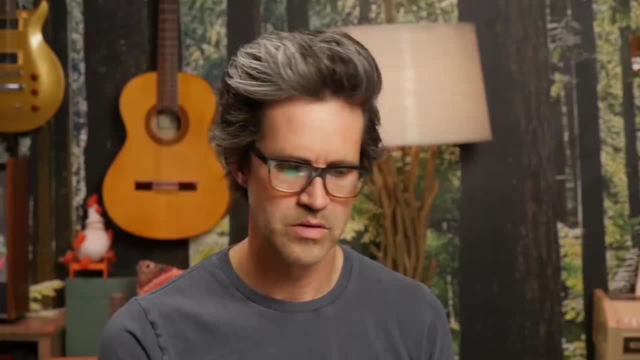 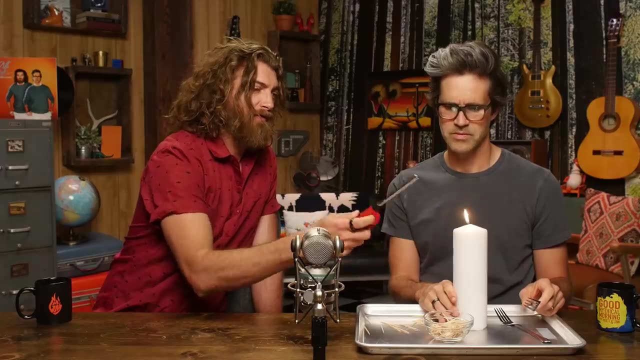 and the fire goes through the smoke. So, like you know this thing, We'll just do that just for just Right, right, right, right, right right, So you get this thing going. Okay, it's going. 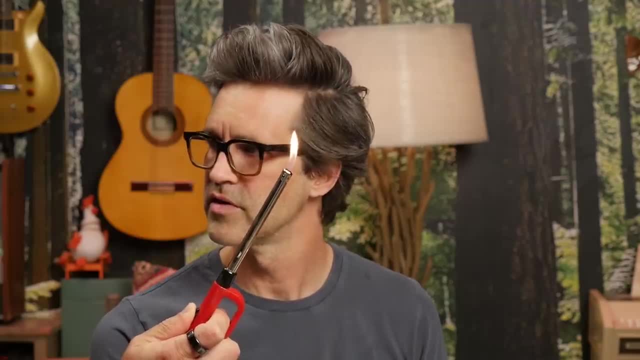 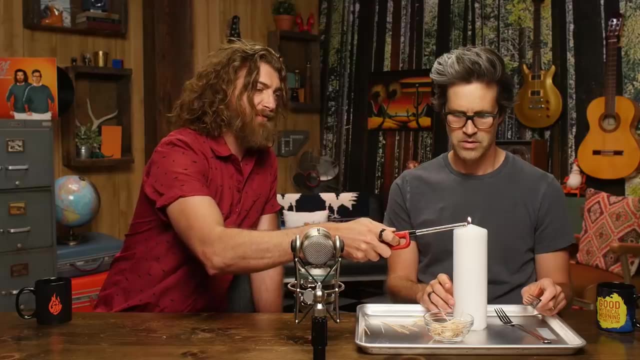 And then you hold on and now blow it out. Does it need to burn a little longer? first, No, And then you light the smoke and it goes back down and relights it. It means the light will go a little bit longer. 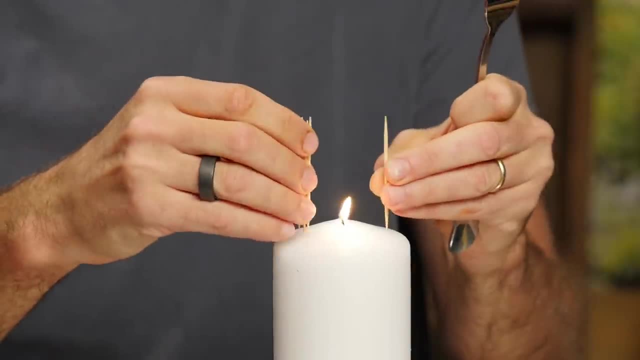 Now that doesn't have anything to do with a fork or a toothpick. If I put toothpicks all around this and make like a campfire, the flame would probably get a lot bigger, which would be cool. That's probably not what they want us to do. 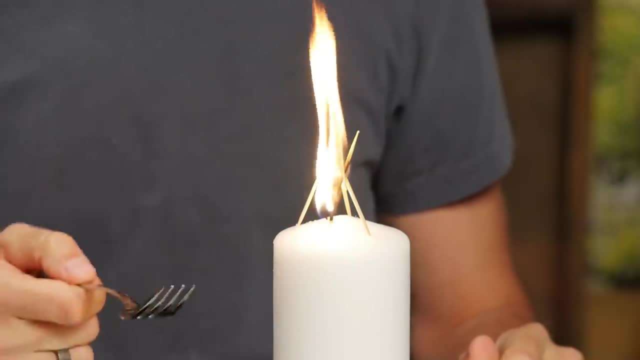 That's what I want to do. Look at that, Stevie. Ah, yeah, yeah, yeah, Is that what you wanted? Put the fork in that? No, I don't want that. Make the fork In fact. please put it out. 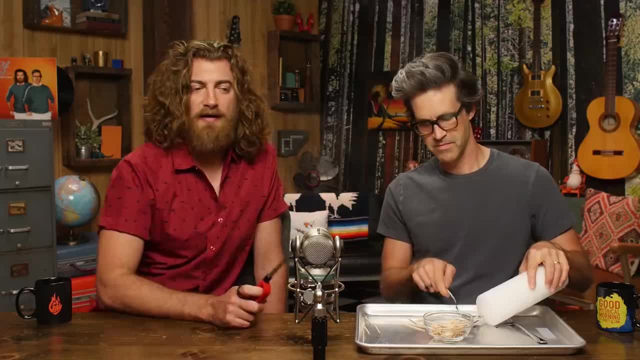 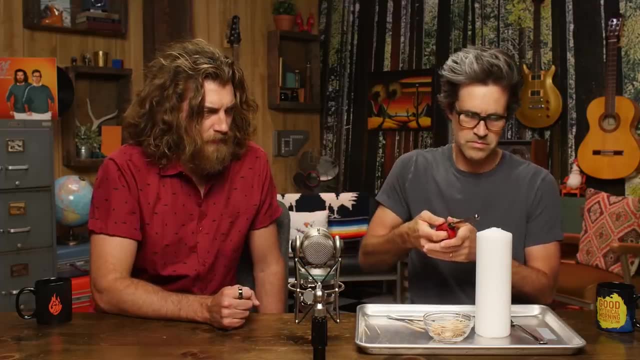 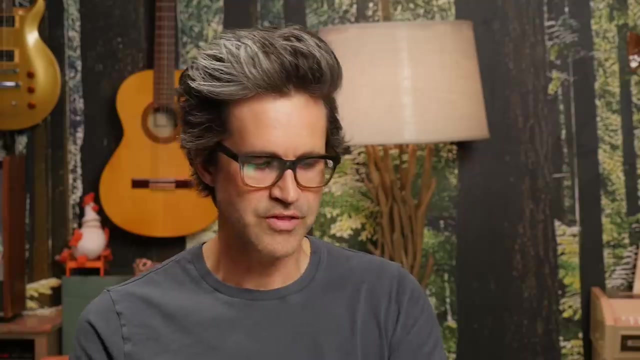 Make the fork hot. Thank you, So that didn't work. Okay, Stevie, we need your lifeline. What are we trying to do here? In this experiment, you will be creating a forking, incredible spinning and balancing act. So the fork. I think we can like put the fork. 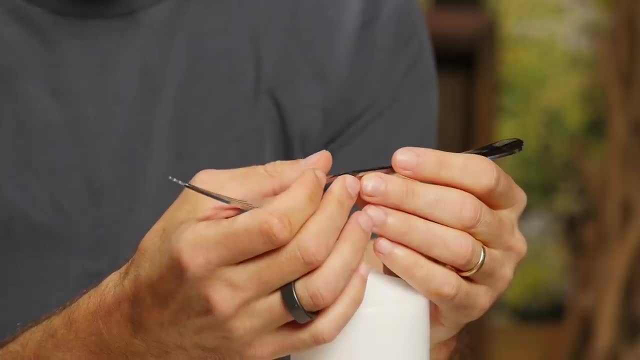 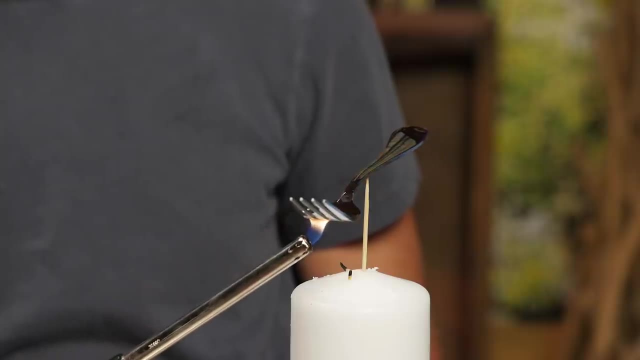 Yeah, Stick the toothpick in the wax. I see people balance stuff on the internet all the time. There you go. Okay, all right, Now we're onto something, And now we just heat one side of this. I'm just going to propel it. 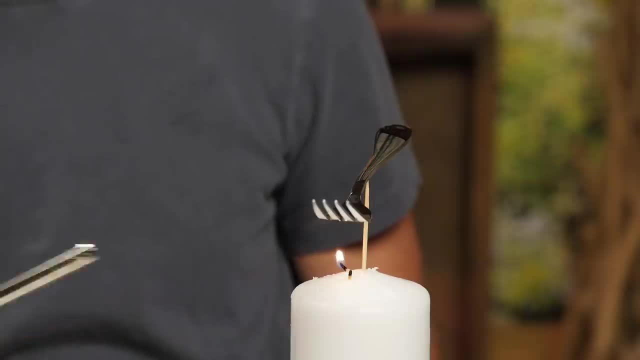 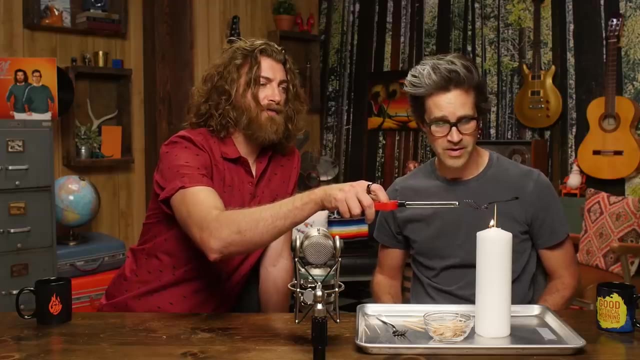 No, no, no, light the candle. I mean that's not going to do anything, But you were impressed that I balanced it on there. Yeah, I can't believe it. What if we put a toothpick on the fork and then lit it? 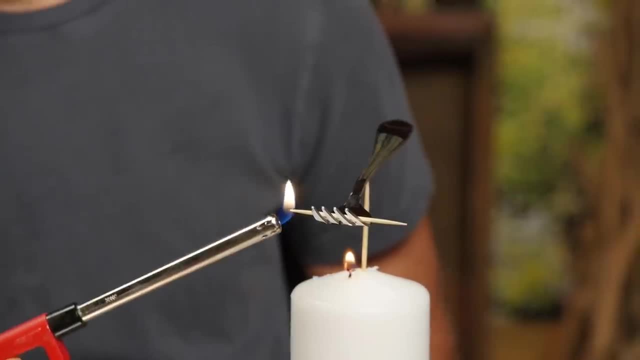 And it's like a little thruster And I light that. Yeah, here we go. Now we're- Got this. We still got two minutes. This is going to work All right. yeah, look at that, We've done it. 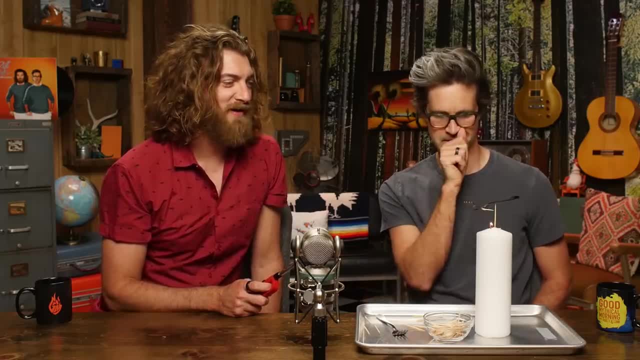 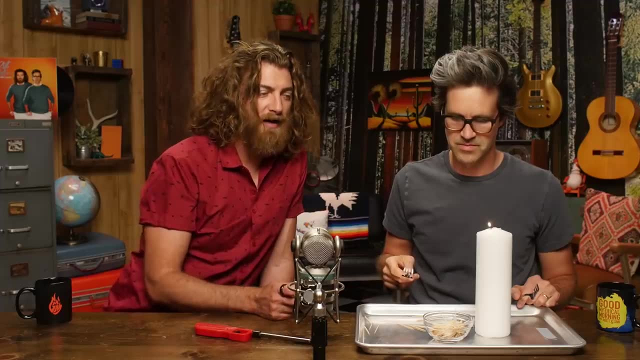 Yeah, yeah, yeah, Look at it, Look at it. thrust, It's going to start spinning. This is how rockets work. Is sticking this in the candle part of it? Is sticking the toothpick in. Yeah, Yes, Okay. so see, I think we were close man. 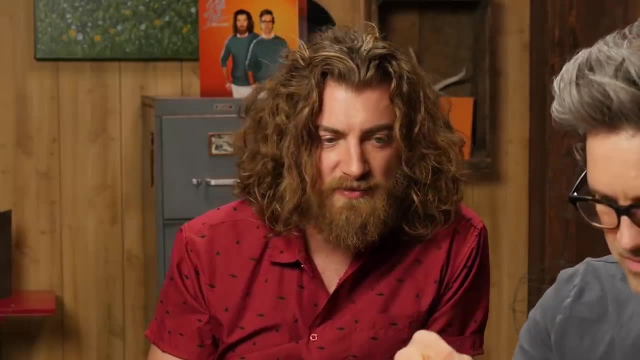 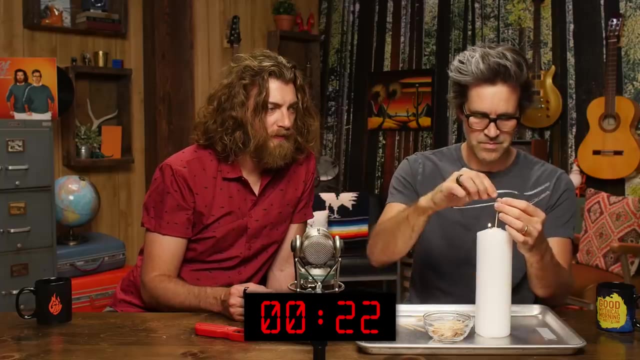 I think that what you're doing with the balancing is right. I just don't know where- And I'll give you an additional hint- You do have to use both forks and you have to do it in 22 seconds. Okay, 22 seconds. 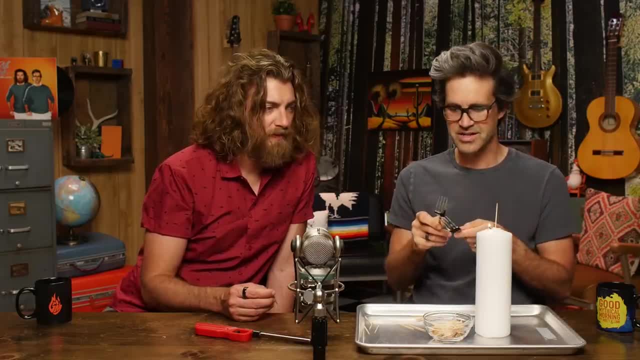 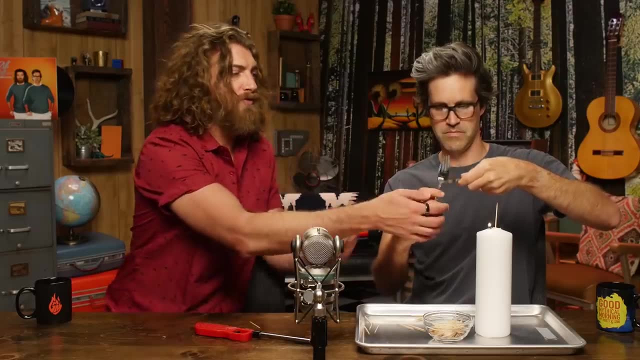 Oh, I think you've got to- Why would they just stack? I think it is like this: Oh yeah, You got to put that, and then it catches itself. Oh no, Oh, oh, oh, oh oh. 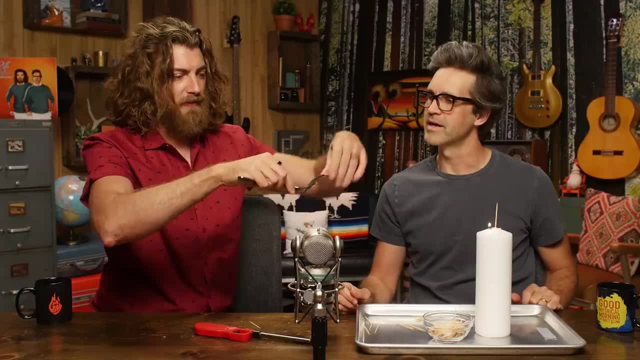 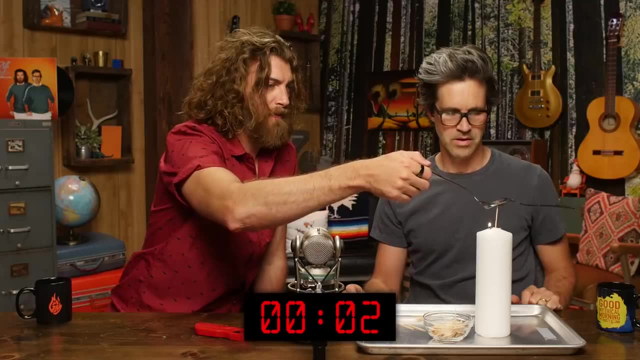 What if you did this? Did this deal right here? Oh, like two youngsters on a date holding hands. Oh, you are so close, but your time is up. I bet you, Caitlyn, can do it. You know what The whole thing will spin. 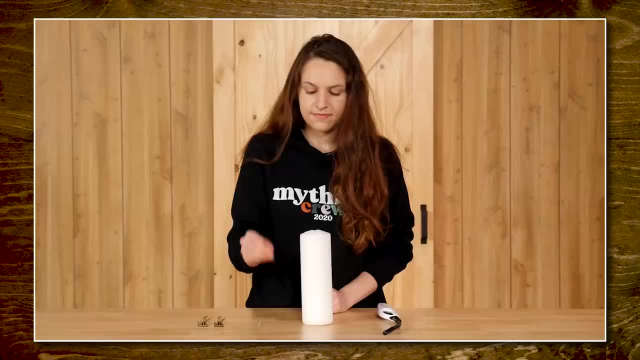 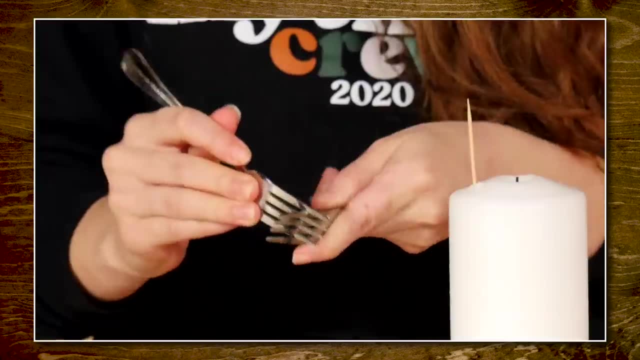 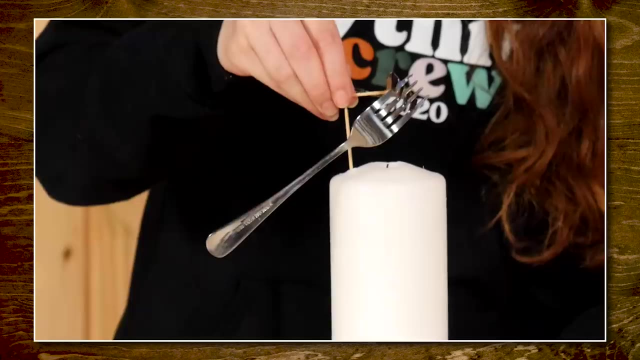 Yeah, let's see what Caitlyn's got Forks on the side. Yeah, see, oh, we got that at the very end. Where does that, where does that go? Oh no, Oh no, Oh no, she did it. 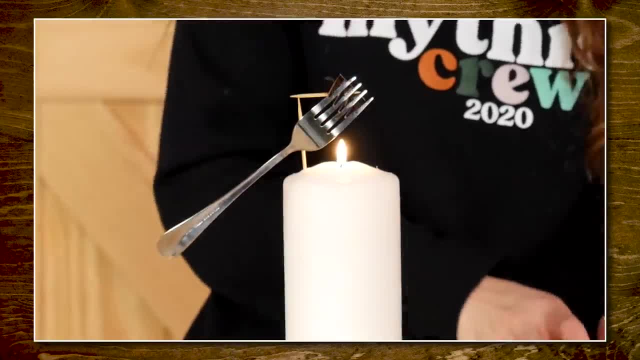 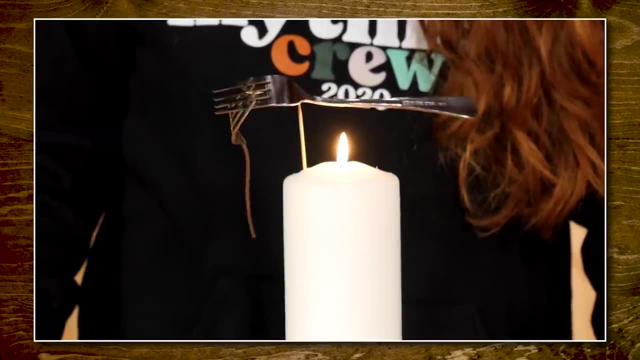 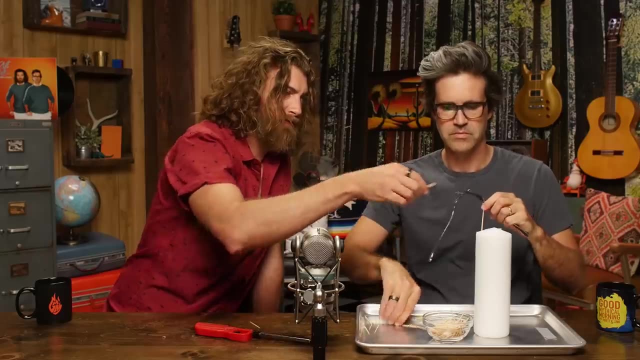